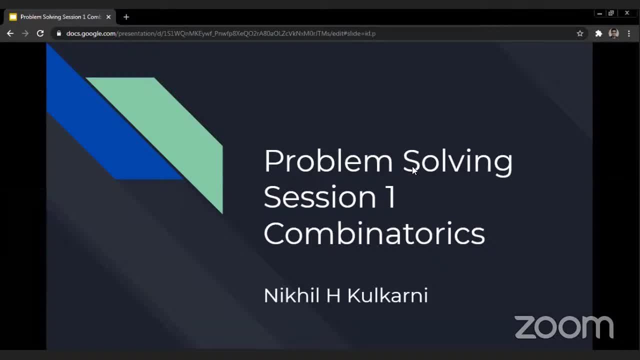 and we want to stay sure that you can understand everything up to a certain highest point so that the problem solving becomes easier. and the problems we will be discussing today will also be of, like PRMO or NMTC levels, and they are quite tricky problems. They are not simple. 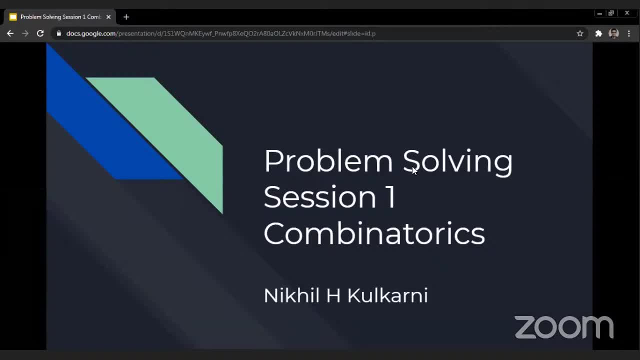 but we will slowly move on from simple to tricky problems. It should not be like that you are solving RMO problems on the first day, the first problem, or something like that. So the structure is somewhat different and I will just provide you with the question. 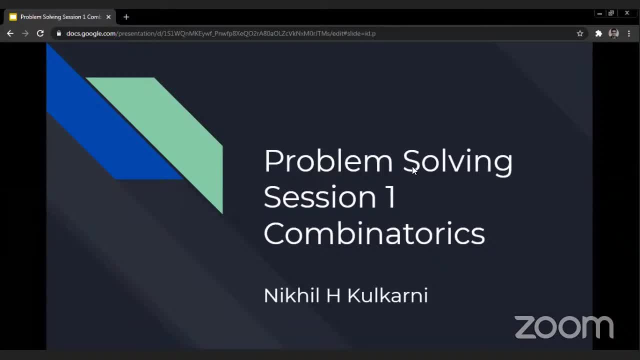 and you have some time to think on it, Then we will solve the problem together and hopefully all of you understand. So I will ask. if anyone of you has any questions, please feel free to ask. If any of you got the answer, then you can ask and answer in the chat, and if I ask you, 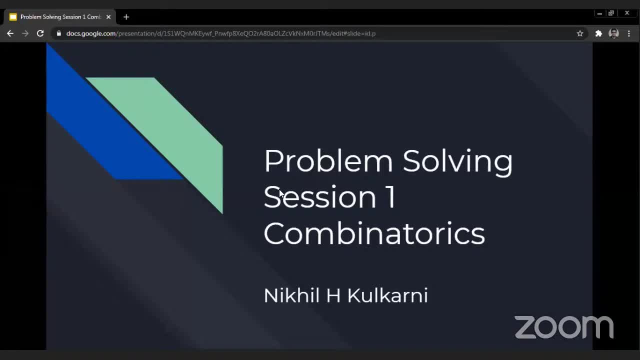 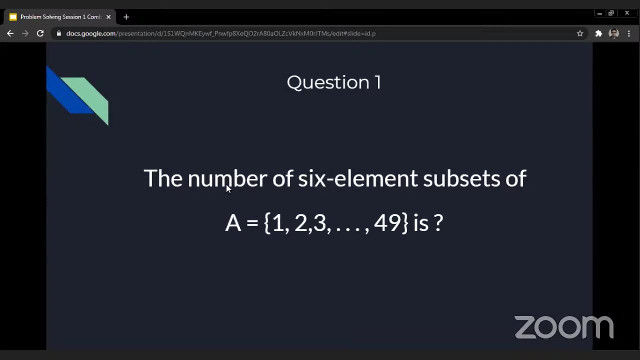 then you can say it aloud if you raise your hand, and something on lines of that. So let's start the session. and the first problem for today- and it's quite a simple problem. Some of you may relate it to what we have done in camp and essentially this forms some 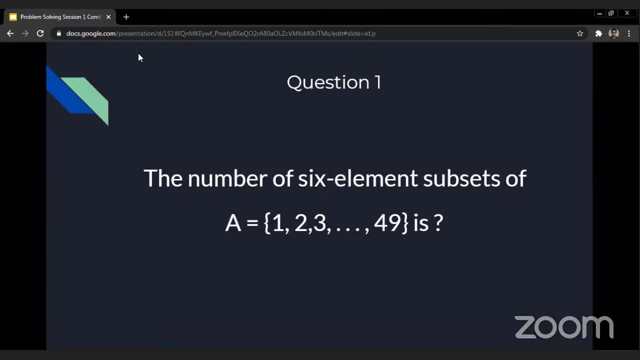 of the most basic principles in combinatorics and I hope all of you have understood it. If you are able to solve it, so just just type out the answer in the chat and send to me or someone else, some other co-host. Let's just wait for like a minute or two for everyone to solve it, because this is quite 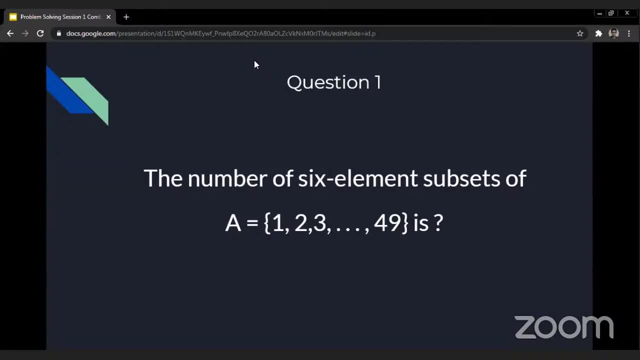 a simple problem And we already have two answers and both of them are right. So I would want others to participate as well. We already have two answers and the others can also send the answers in the chat to me or to Imran, so that we can check whether your answers are correct. 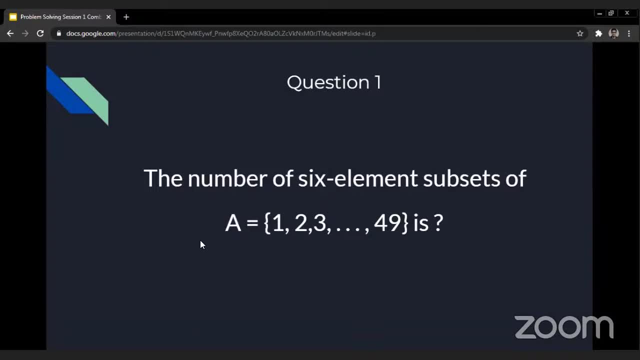 And the answer is quite simple. This is a really simple problem, but the implications Are quite different. So this can be stated in a lot of ways, and it's it's just. this is in its raw form. This is in its most raw form. 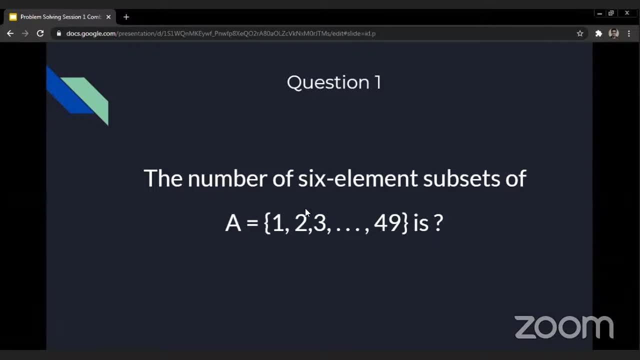 So you can, you can add any layer to it, any cover to it, and this may appear anywhere. But this is a really simple question and we'll we'll be moving on lines of these, So it's not like we'll have all the questions like this will will go to a really high level. 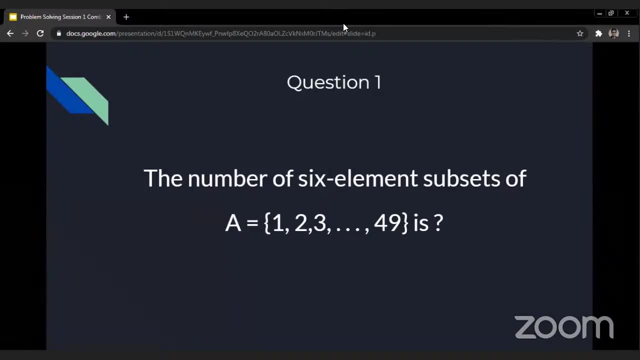 problems quite soon. Okay, we have three answers now and all of them are right, Yes, Okay, so I guess we'll we'll move on to the solution. Does anyone else have any solution? if yes, then they can put it out in the chat to me. 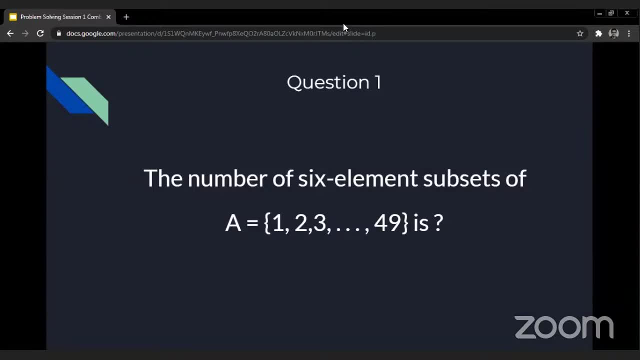 or to Imran. Yes, so Tanmay, Samyak and Archit, all of your answers are correct and, according to what you have put to me, the method is also right. Because this can? this is actually resolved in a really simple way. 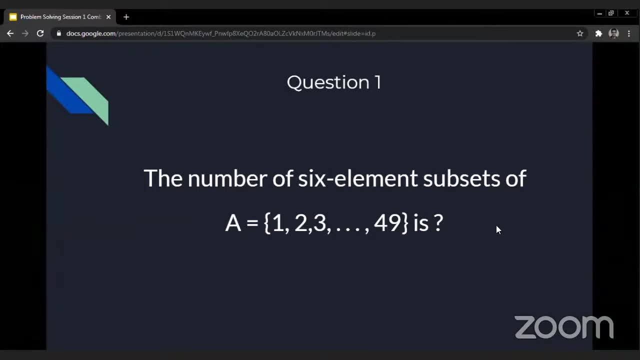 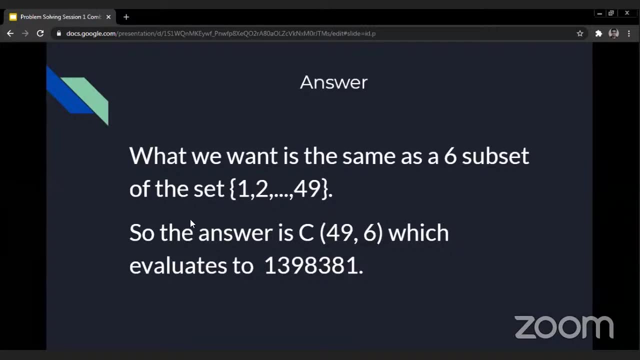 So we can move on. let's let's move on to the next, to the solution. actually, and according to what we had discussed in camp. I find it relatively, relatively simpler to explain to all of you in this way. So what? what we have been asked to find is just a six subset of the set of integers one. 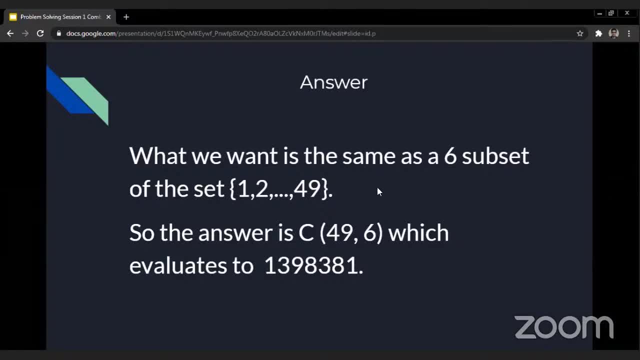 comma two, and so on till 49, and this, this six, subset. We know that the number of subsets are subsets is n choose r, and so this problem can simply be answered as 49 choose six, which is the same as 139, 8381 or I guess something okay. 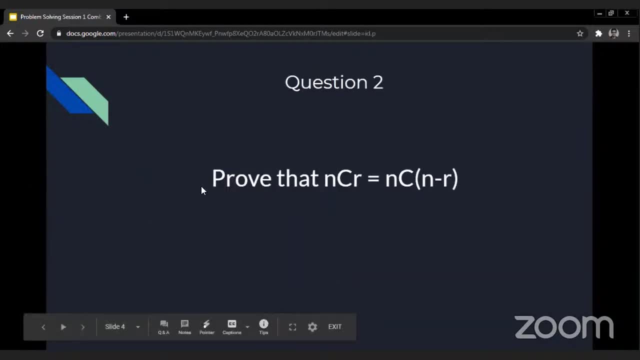 So let's move on to the next question, And we have already seen this. if, if you guys remember from camp, This is quite an important identity and it's used everywhere in combinatorics. This is, and it has multiple solutions, It has multiple methods of two and we'll be looking at three methods. 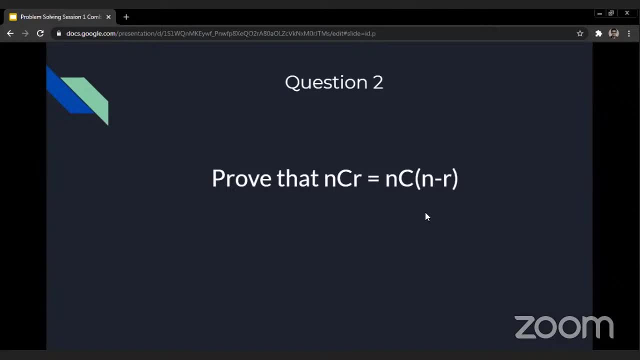 But I want all of you to do this, and if you can, just just type it out in the chat and send to me, or else I'll ask you to raise your hand and just tell the solution, If you can try to type it out, and till then others may also come up with the solution. 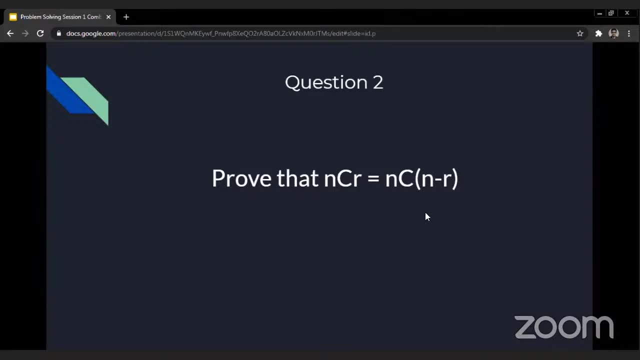 Okay, that's great, And so if you can just type out one and till, then maybe someone else who doesn't know of the solution before he or she may try the solution. So let's, let's give this a minute or two. Yes, that would be right, Samyak. 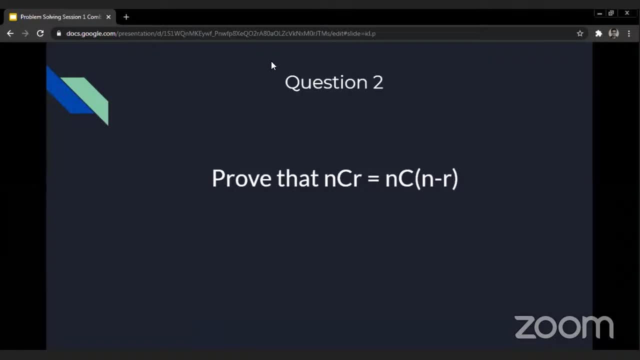 That's one method, That's one way we can think about it. Right, Samyak, right? So what we have up till now is we have got two people giving us two different solution, and that's nice, but I would. I would want others to participate in as well. 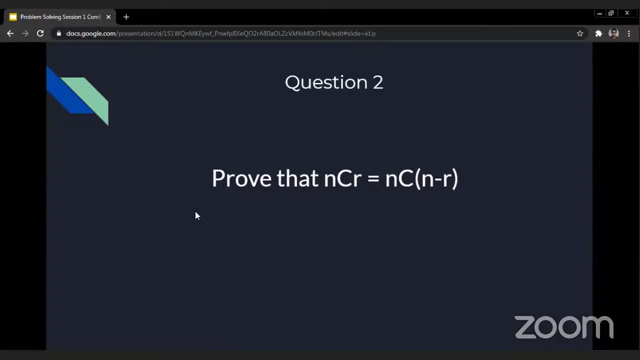 So that would be more fun, Right, Archit? Okay, Aditya, I did not quite understand why by replacing R. why? why can we replace R by N minus R? So I want exactly this: Why can we replace R by N minus R? 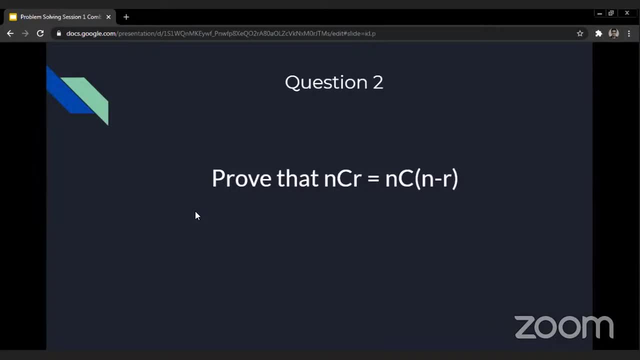 That's that's the question. Okay, okay, I'll. I'll check it. Aditya, I want you to tell me why we can replace R by N minus R. Right, If this is NCR and if we replace this by N minus R, we're going to get the same thing. 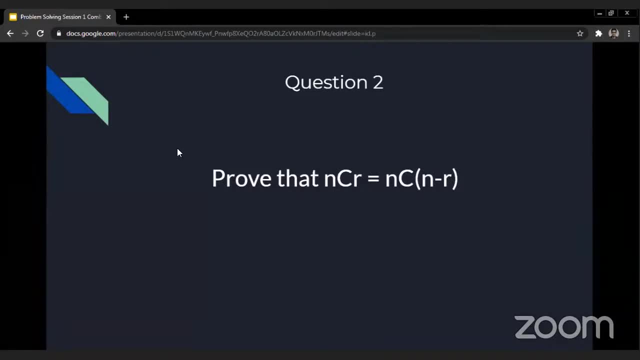 But why? Right, Right, Aniruddha. So this question we have got a lot of people solving and and that is quite nice. Yeah, we get the same thing. on algebraic evaluation, we evaluate NCR, then we get the same thing. 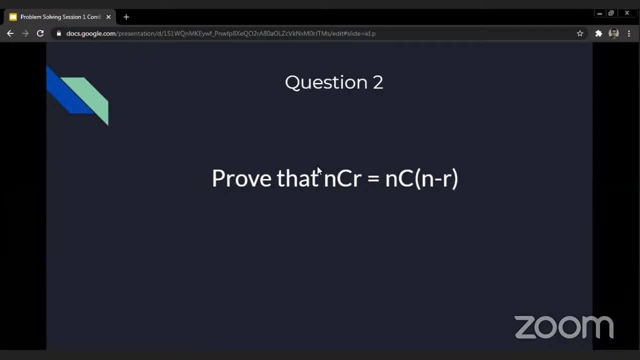 But it's not. It's not that We can. We can. We can simply put in N minus R and R. These are interchangeable, but that's exactly what we need to prove. So if anyone wants to put out their solution in the chat, that this would be the last minute. 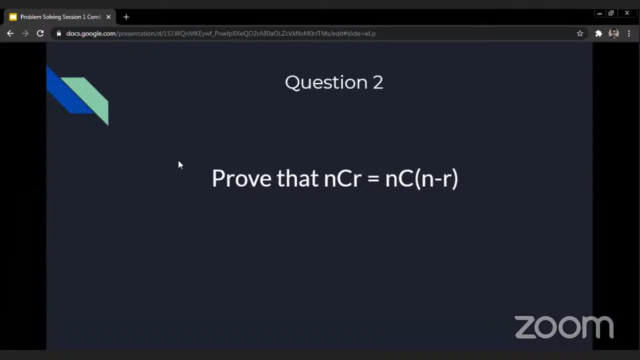 or so that they can put in. Yes, Imran, I actually had planned that. Right, Tanmay, Right That. that is what you have sent me. That is the exact logic of why a newer type of proof works, And I'll just give you a glimpse of it. 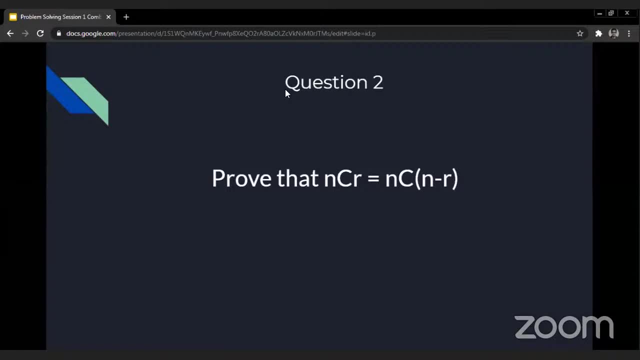 Maybe we can have. we can have another session on it completely, And it's quite interesting to see how this logic can be. can be, Can you be used to generate a newer type of proving technique? OK, I guess now many of you might have tried to solve it. 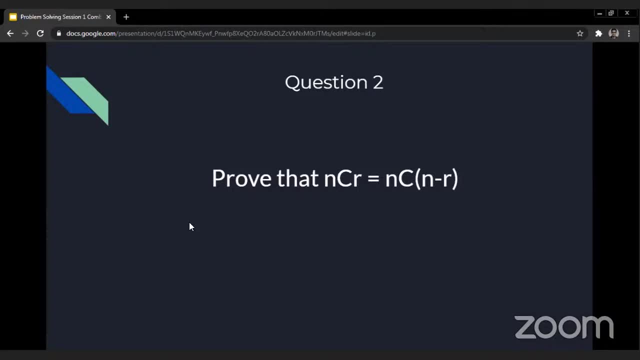 I'm still expecting replies from other people. I hope that you all are able to solve the questions. I don't think we are moving at a at a really fast pace actually, because these are quite simpler problems, but they are fundamental. So I don't want any of you to have any gaps in these. 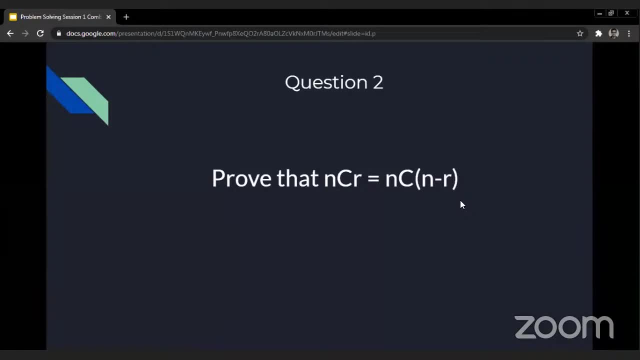 And OK, now let's, let's go on, Let's move ahead to this solution. OK, so we can. we can solve this method actually by three ways. I have already told you. the first method can be algebraic evaluation. We know that, NCR. 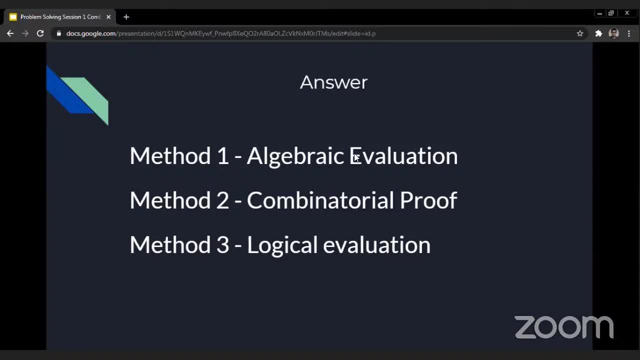 Is N factorial divided by R factorial times, N minus R factorial. And what when we evaluate both of NCR and NCR and minus R? so that that would lead to the same thing algebraically and that would be the simplest form of proof. Then the other thing is a logical evaluation. 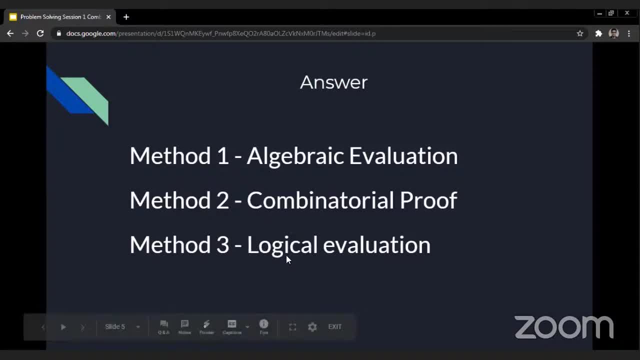 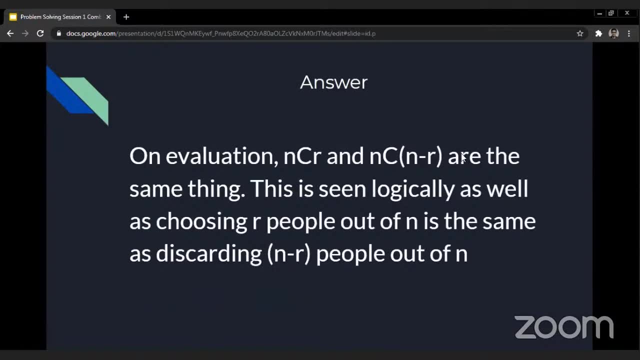 And this actually forms the basis for combinatorial proof And the logical evaluation will. will move on to that in a second And OK, So the first one is the one evaluation and NCR and NCR minus R are the same thing. And what, how can we visualize? is the logic logically, is that when we are choosing R people. 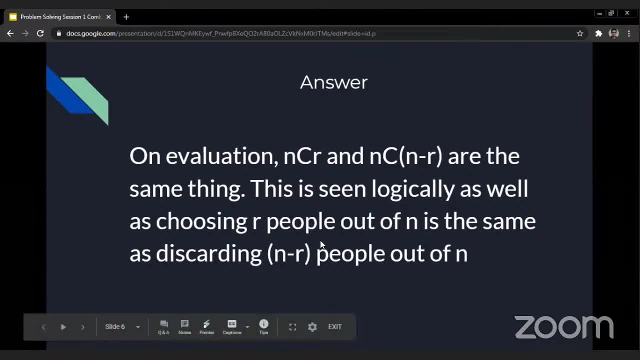 out of N people. So essentially we are, we are choosing N minus R people to discard. So if you have N people and you want to choose, suppose, one person, then actually what you are looking at is you or you want to, you want to remove N minus one people, and then you 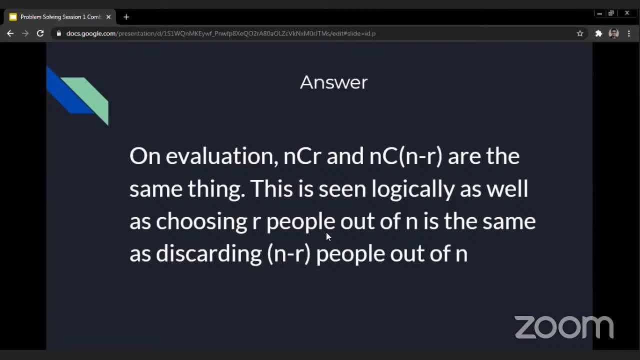 will get that one. So you can think of it in two ways. and that that this logical evaluation is the basis for what we call as combinatorial proof- And I haven't given the combinatorial proof here, I just mentioned it. And what combinatorial proof we can give is based on the same logical evaluation and combinatorial 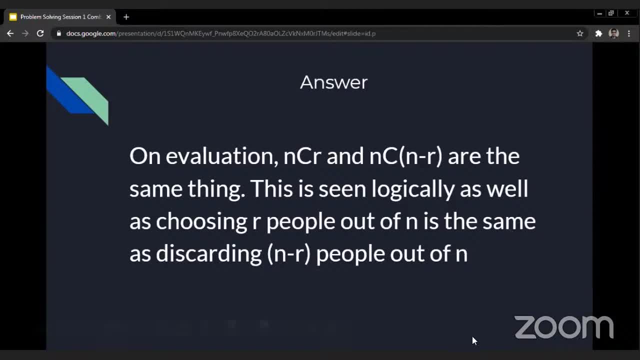 proof. What we do is we ask a question and we get answers to it using two methods, And, as the question asked is the same, therefore the answer must be the same, And so both of the sides must be equal, And that, And we can move on like that. 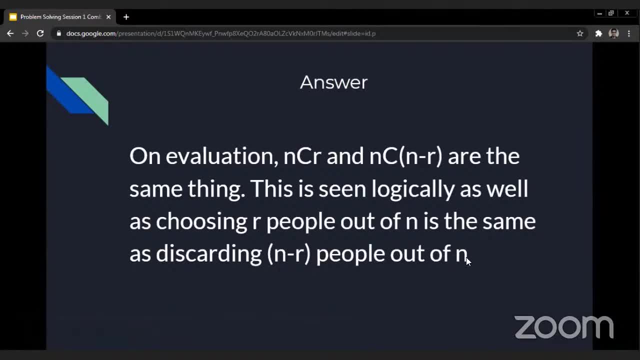 So I hope all of you, all of you are getting what what I mean by discarding N minus R people out of N people, because this idea is quite important. So I'll repeat it once again: on algebraic evaluation, we get that NCR and NCN minus 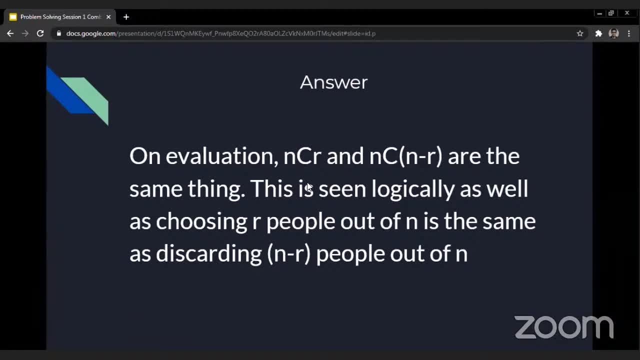 R are the same thing And it's. it's just in the form you can. you can just substitute in the formula. But why logically? So you must have a Y side of it, And that side is explained by this in this sentence earlier that we are choosing our 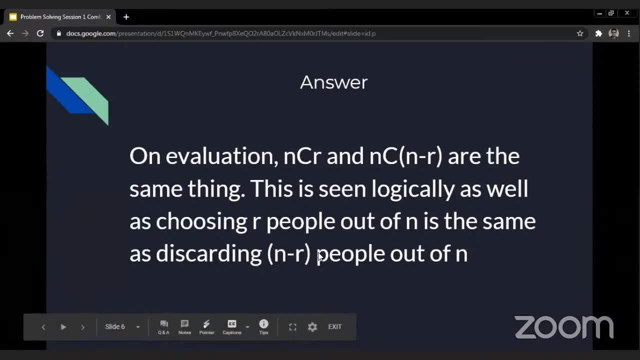 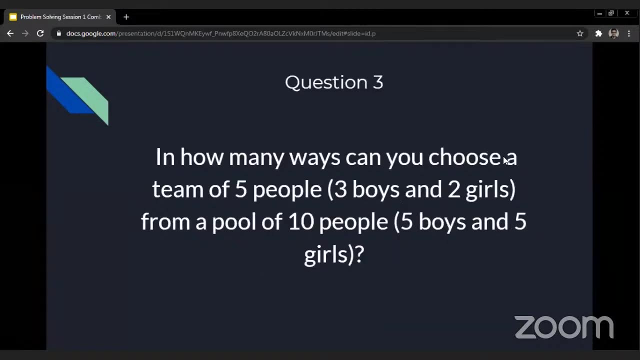 people out of N people. that is, we are discarding N minus R people. or maybe we are discarding our people when we are choosing N minus R people. Okay, so now I think let's get to the next question, And I guess for the next question we'll have some time. 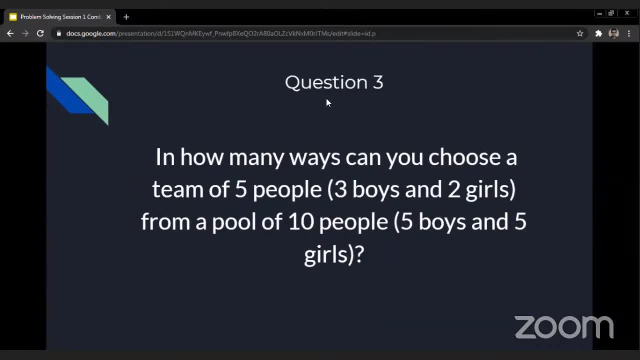 Even this sort of question we have seen earlier, when, when we are discarding N minus R people, we are discarding N minus R people. So we are discarding N minus R people. So we are discarding N minus R people. Okay. 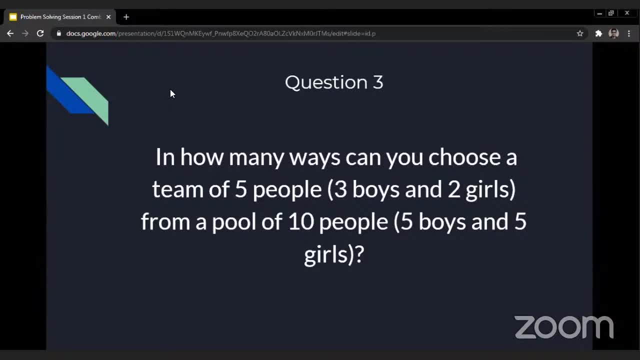 So wrong, because this is a little bit這樣. We are Yes, Okay, okay, perfect, Let's wait a little bit minute to solve this one test, let's do it. So then we should have done it obviously at add. 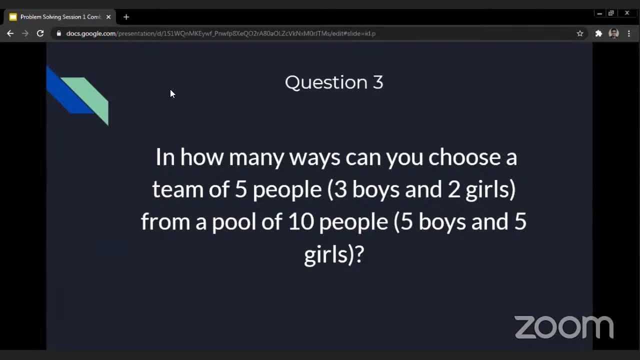 And then, instead of adding some stress on that we had done can and in camp I had, I had explained the solution. We need to take a lot of time to think out first, but even I was unable to solve this question sometimes ago. but if you think about it carefully, then there is the logical side. 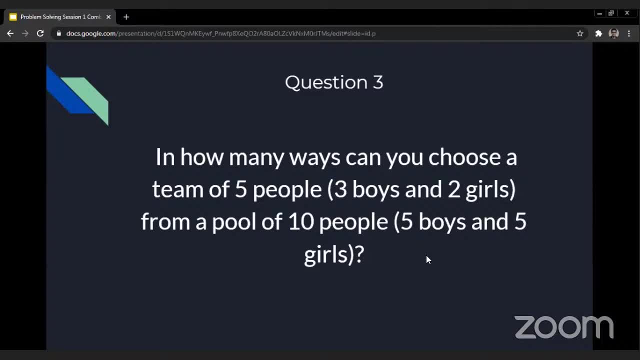 to it not be that hard, okay, so go on. now. you have around two to three minutes maybe for solving, okay, so I have different answers this time. okay, turn my. that is right, some milk does it evaluate. to wait, let me check once. actually I don't get how you get, how you got your answer, so it would be great if you can. 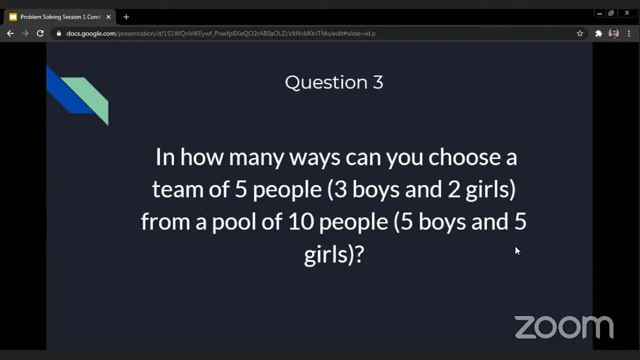 type out in the chat and tanishq, even you, I did not get how you got your answer. it would be great if you type out in the chat and just just tell me how, how you got your answer, explain it in terms of combinations or permutations, maybe, and if any of you have any doubts then you can ask. you raise your hand and 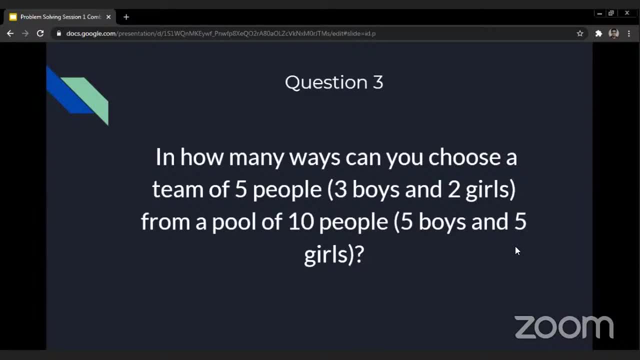 ask your doubts, any doubts in the question. if there's something missing in the question, you feel that the question is not clear, you can raise your hand. you can act just with me. sorry, I guess that one answered rescued institutions- evaluation part. okay, so this is correct. sorry, I guess I have made a mistake in my solution. just evaluation part, okay. so I've got some different answers than my. how can it be? that's right. that's right. or if an morbid and tanishk, I want you to revise your answers now. answer is quite close, but I don't get. yes, okay, that's right. I have asked you to revise your answers. the answer is quite close, but I don't get. yes, so it's definitely correct. but at that I don't get this right. but it is correct. yes, that's right. 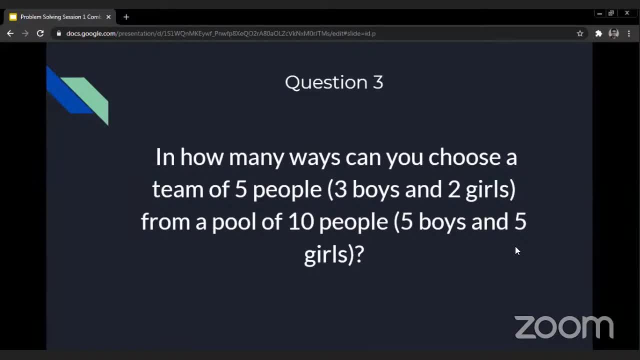 so what we'll be using to solve this question is just, uh, simply combinations and some multiplication rule thing, maybe the answer. i guess you, you made a simple mistake or something like that, because the what, what you have got, is maybe uh, due to, uh, yeah, okay, uh, aditya vardhan uh. 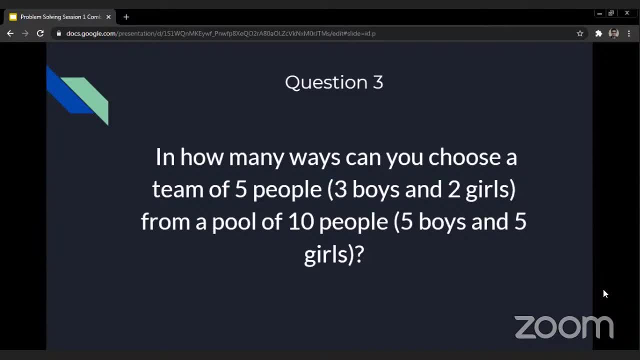 let's see uh 10. okay, right, aditya. okay, i'll have to call both of you uh, aditya. your answer is right, aditya vardhan. i think you need to revise your answer. i i think i know where you are stuck. 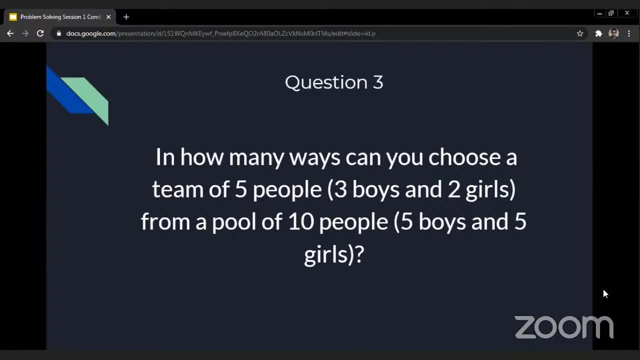 uh, because, uh, that can be quite of a uh problem. okay, so another minute, just this last minute, for everyone to revise and send their answers. i want, uh, aditya vardhan, then um tanish and aniruddha. all of you can revise your answers because they're not quite. 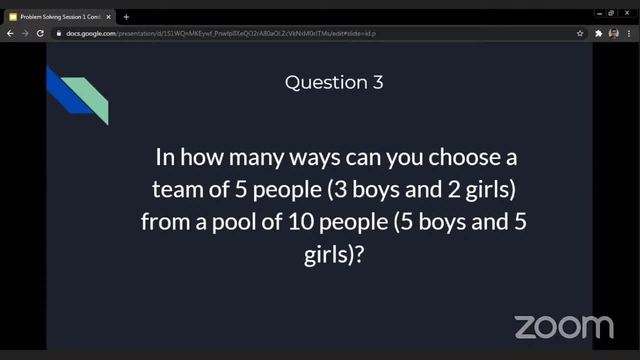 clear. i, i want, if you can, if you can, then just just tell me how you got your answer, so that we can, we can get to know, uh, the thing that you're missing exactly. uh, that's right, vedashree aditya, i think you're missing out on some some. 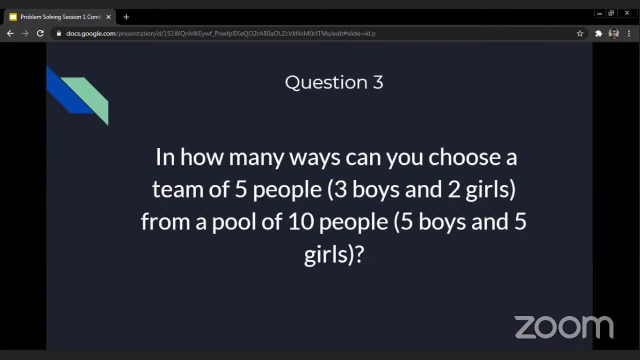 minor point and uh, let's see, the answer is still wrong, although i guess you are quite close, but uh, not, not algebraically not. uh, not on the number line though. okay, so just let's look there so that, uh, i can actually see you. uh, you were on the number line there a little bit earlier than i was going on a second�. line, but i don't understand your situation. what's the question is? i haven't really got any thing to mention, although i think that i can think of very closely sleeped down anyway. so if you can get this from your question in your waterpacks frequently too, is it good for computer, and may well. let's see, this is still wrong. 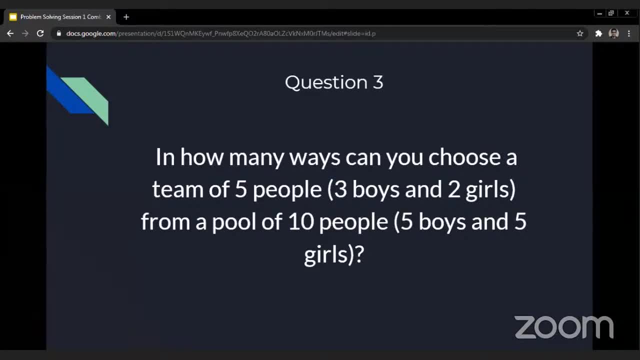 just 20 more seconds. i guess now you'll start getting a feel of how the problem solving session will be. it's like a competition for all of you to send in the answers, but it's not. you should not stress too much, but you should. you should think of it playfully like it's a sort of competition, but less. 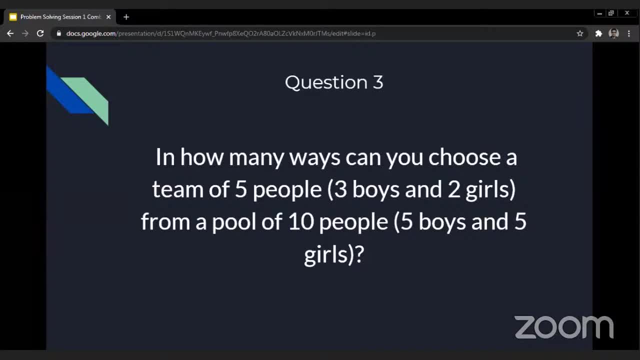 competitiveness. it should not be. you're competing against each other, but it's sort of a contest, maybe. okay, so now i think we can move on to the solution. uh, no, i don't think it's. it's that, let's. let's get to the solution and we'll find out what, what. 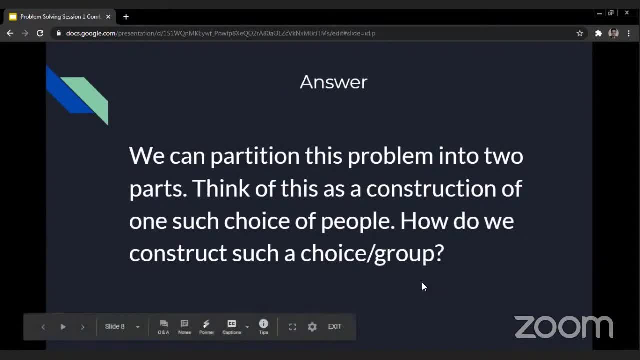 got you wrong. okay, so we have done this type of problem, uh, in the selection camp, and we have done this type of problem in the selection camp, and we have done this type of problem in the selection camp, and this is why i had asked all of you to go through the videos. 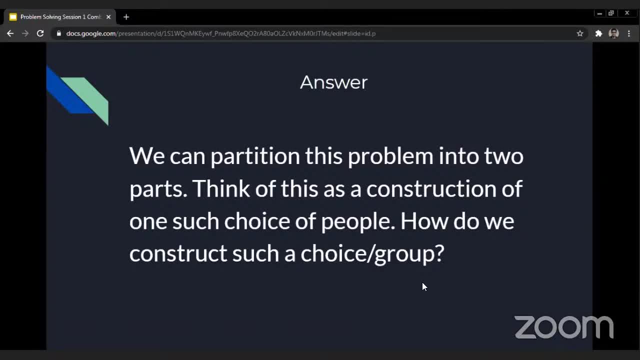 because such problems can come in different ways. they come in different altered forms, but essentially it's just the same thing and half of combinatorics is just understanding that it is combinatorics and that's what gets you wrong most of the times in olympiad and maybe we can. we can. 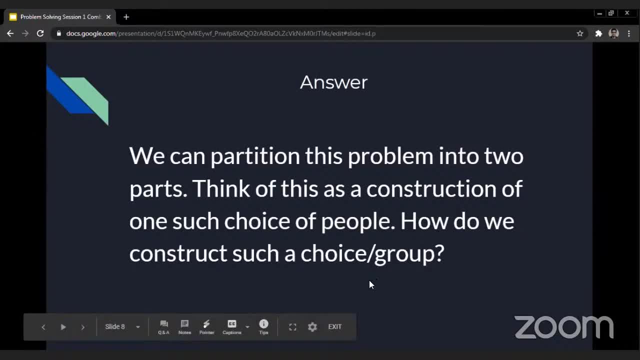 have such a session because, uh, half of the times, you don't know what to use. so, uh, this problem is partitioned into two, uh, two parts, and i like to think of it this way because, uh, it gets your mind cleared up, uh, so, as as we had done in camp, we need to think about it as a construction of, of a choice. 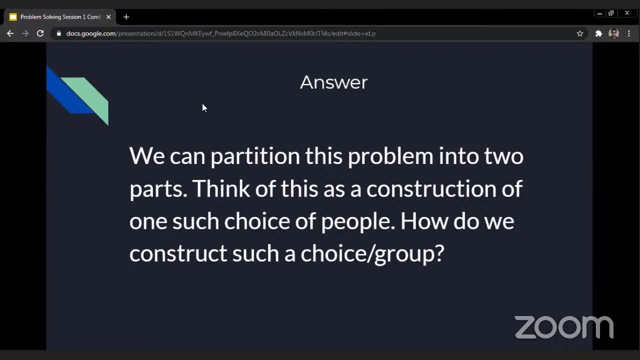 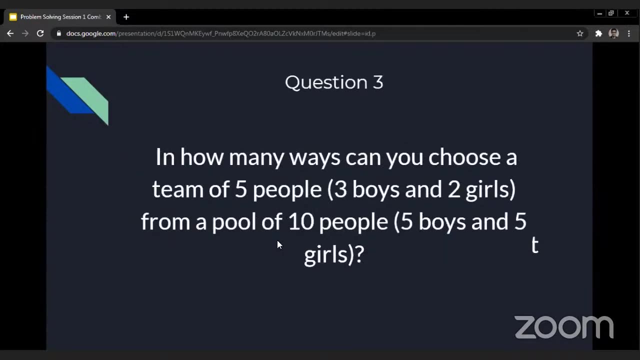 of people, of a group, and how? how can we construct the group? so we, we do it in steps, and what? what can you give the first step as? so, let's see, the first step will be to choose a boy, because the problem us us to choose a team of five people where there are three boys and we can choose. 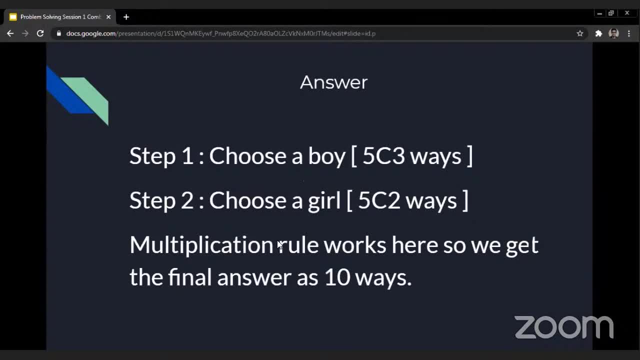 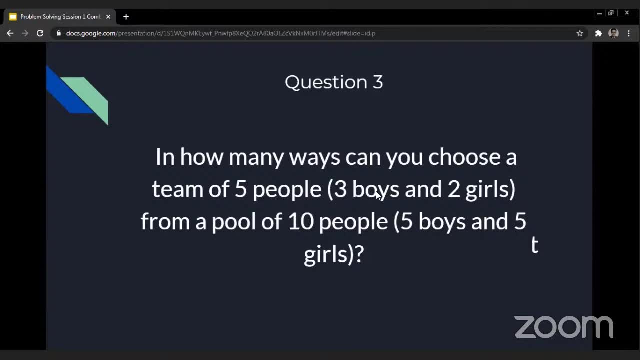 the boy in five. choose three ways, and that is because we have five boys. as you can see here, we have five boys and out of them we need to choose three boys, so there are a total of five. choose three ways to do step one and we are thinking: 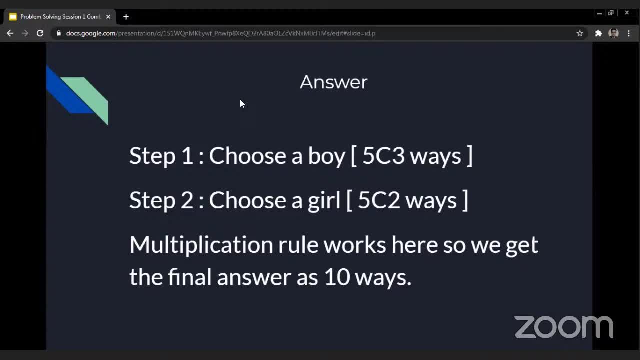 about it this way so that we can use the multiplication rule. so keep in mind, if, if you you see such a problem, you can use multiplication rule and for that you must partition it into such parts that they are independent, and is not okay. so for the boy, we have five, choose three ways. and for the girl, we have five, choose. 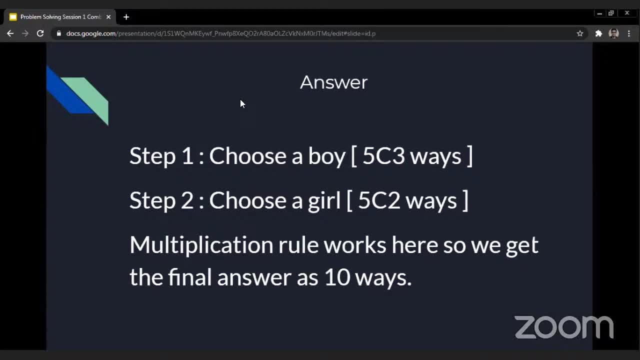 two ways, because there are five girls and we need to choose two of them for the team and I haven't asked for the permutations of the group, so it doesn't matter right now- and by the multiplication rule, this should be 100 actually, and that was what I was talking about earlier. so 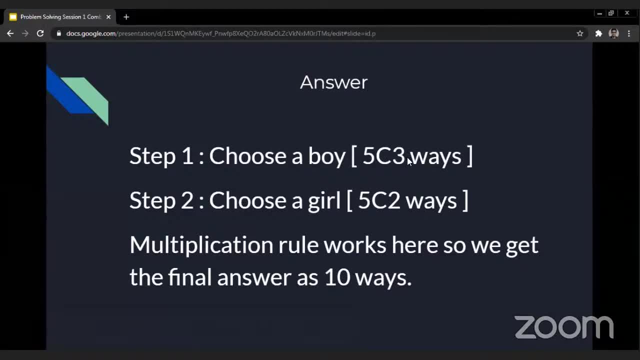 by the multiplication rule, we get this as: five choose three is 10, and five choose two is 10, and it should be 10 times 10, which is 100. so the final answer is 100 such ways. okay, let's. let's move on to the next question, and for: 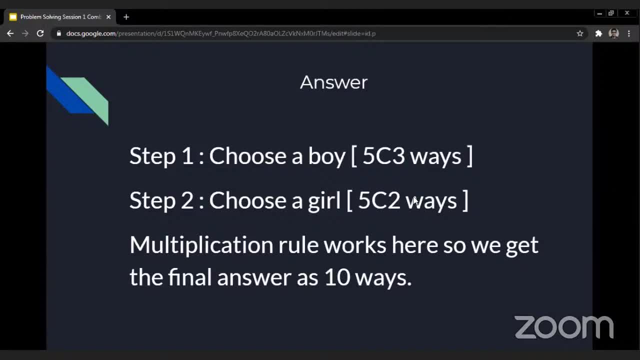 those who did not get. is everything clear or is it not okay? and you know? the right option in terms of your? my perspective is that: do you want to manipulate this $1000 per day or something like that? so get more money and enter that all these time groups. there is so much range you can, you do. 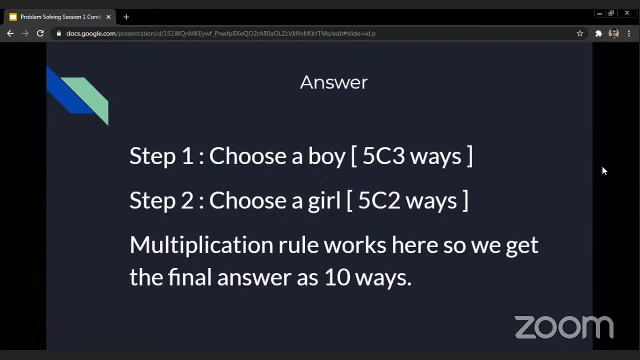 it once. there is always challenges, so you can have that control and the sharing of the money. there is no use in it. so now here is the question: will I get more money? and then what will be the cost? how will we get this return here? what will be theill difference of your carry, your shopping? you have to do it all. 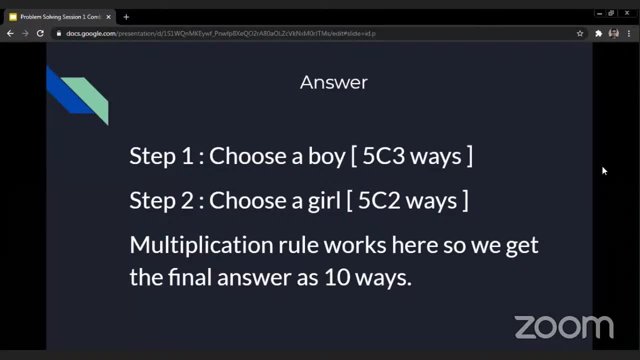 much easier to solve. so now, if everyone has understood this problem, put a yes in the chat to me, like some people have already done. just put a yes, okay, cool. so now we'll we'll get on to some quite higher problems and they are not simple anymore, so you cannot think of them as simple problems, but they will require the basic thinking. 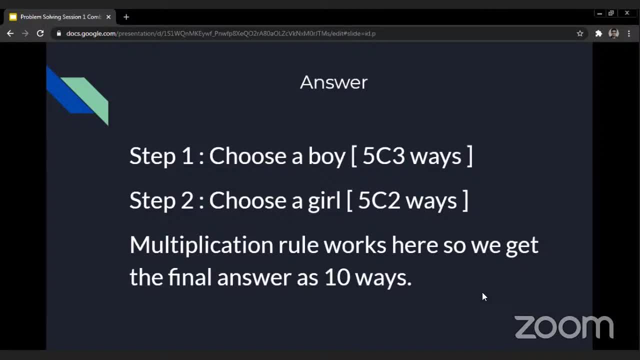 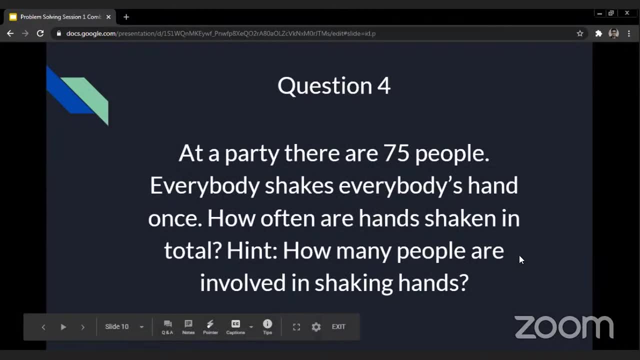 that we have talked about. so for the next problem: okay, even this is a simple problem, actually. let's see how many of you solve this. first. i think i'll give around two to three minutes for solving this problem and then we'll move on and if you get the 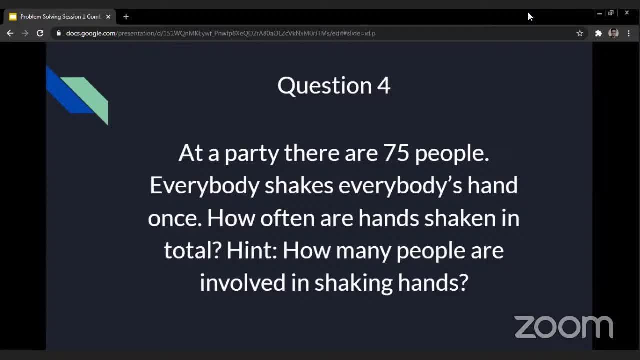 answer, post it in the chat to me, or imran. okay. so all right, i think that was good enough. we're gonna move on now and i want you to talk to me about this problem. who are you talking to right now? oh, so you're talking about. did you get the answer? 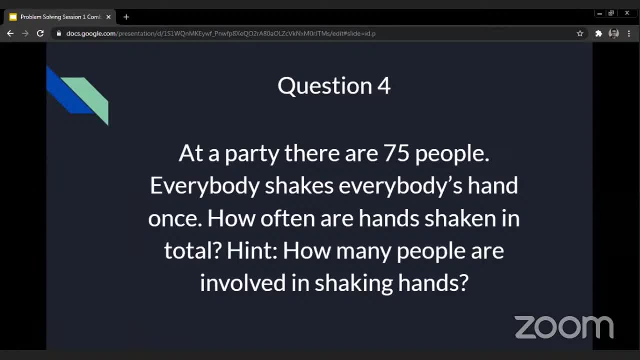 yeah, so we're going to do the same thing. so first we need to talk about: the question is: how do we solve this problem so we can get to the bottom of this and we can get to the bottom of the problem. that's why we're gonna be using like this: 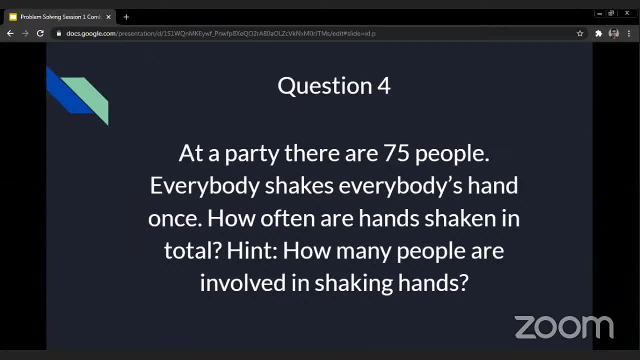 so the question is: what do you mean by the answer? i'm answering the question, okay, and so this is one of the first questions. the first one we're gonna ask you to do it is: could you, or some of you, know of one or two? you, okay. so i have been receiving some, uh, some answers, and let's see. 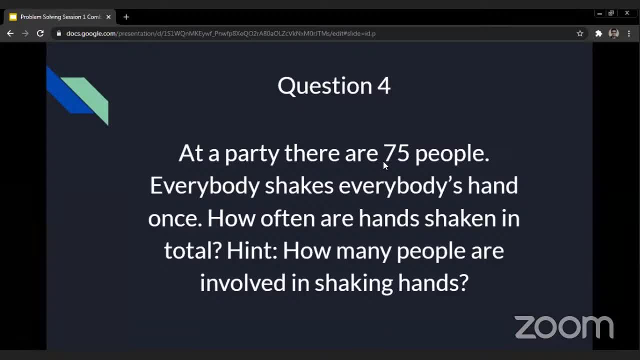 oh, okay, uh, first of all, um, i have received two answers from lot of people, so the first answer is 2850 and the second answer is 2775, but i don't know which one of is is the correct answer, because the answer that i have 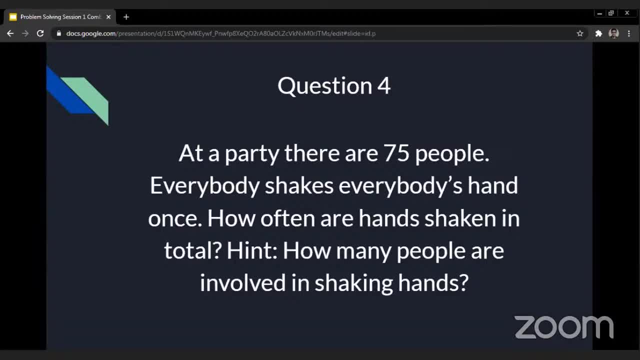 is in terms of, in terms of choosing, in terms of combinations. so i'll have to evaluate it, but i don't have access to it right now. uh, let's see. uh, samyak, your reasoning is correct and i just want you to explain to me this in one particular combination term. 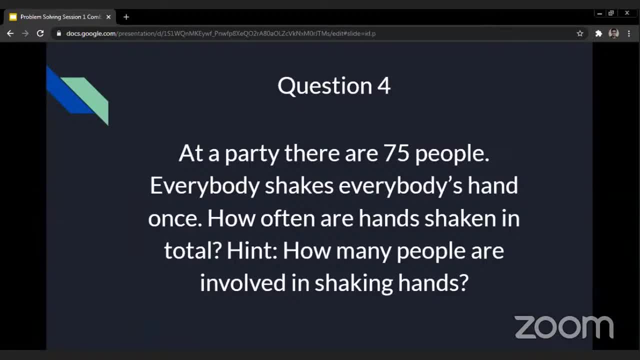 okay. so, uh, your reasoning is: uh, right, and aditya vardan, it won't be 74 factorial. oh no, no, it's, it's countable. oh no, no, it's, it's countable. it's not that high. you know how high 74 factorial you can't even count like 20 factorial on a. 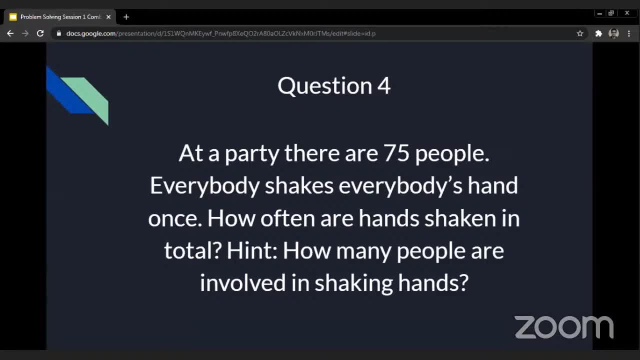 calculator, maybe not even 18, 18 factorial, it's it, it's. it's such a asymptotic function like it. it goes really fast to infinity. okay, akshat, sorry, archit, i think that will be right. uh, yeah, you use the right reasoning, but you can also think about it in terms of combinatorics. 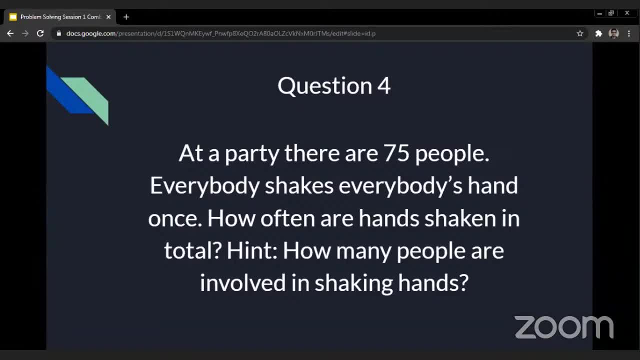 actually, it's quite related, uh, to triangular numbers. okay, so the thing is i don't know the actual answer. i know it in terms of combinations. that's what i've been telling you. okay, so the new answer i've been getting from everyone is 2775 right right than my right, samyak. yes, uh, tanishq, i want you to revise your answer, it's. 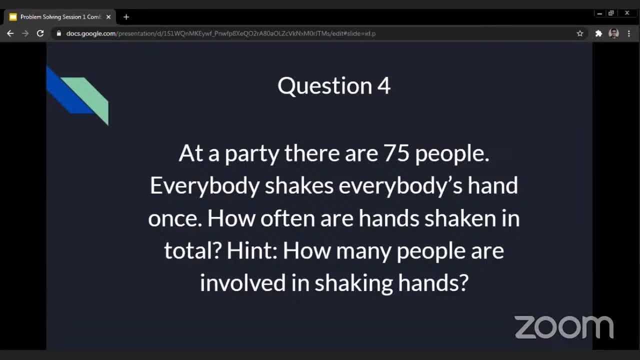 it's not 407, uh, by far. i've received the answer, that is 2775, which i guess is 2775 is no, it won't be 74 to 73.. it won't be 74 to 73.. you don't want to choose 73 people for a handshake. 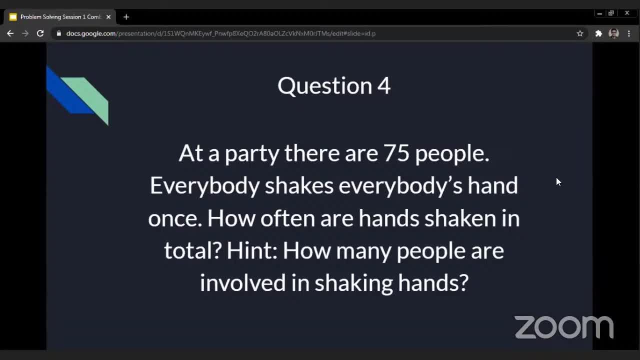 okay, i'll, i'll, okay, okay, okay, okay, right, vedashree, your idea is right, i guess. now just give me a minute to think about it. just give me a minute to think about it, okay. so this problem requires you to think in some different way. oh, that's a great fact, uh, samyak has. 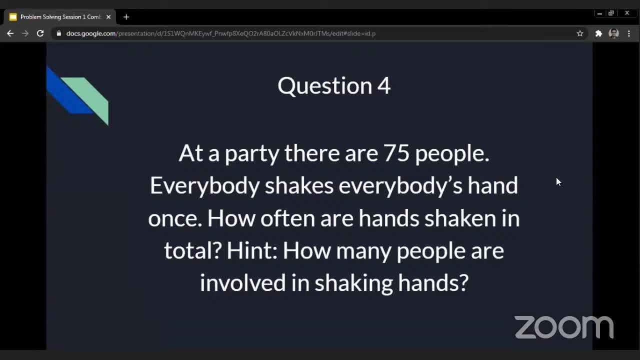 sent a message saying that 74 factorial has around 103 digits, and it may be true because of the factorials. oh, that's correct. that's quite a lot, whoa? okay, 109 zeros. so we are getting around 100 zeros in 74 factorial, right, aditya, that's. that's exactly the logic that you must apply and you can apply it in. 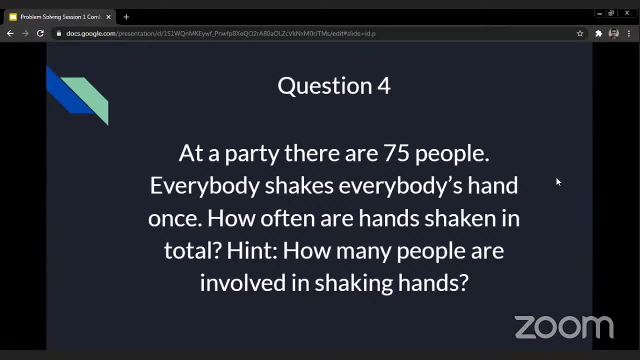 terms of combinatorics, or you can apply it in normal answer. yeah, uh, yes, imran, that is the correct answer and the people have been sending me, uh, it evaluated terms, so i don't actually know, but that is the right answer in terms of what i know. aditya, your idea is correct. 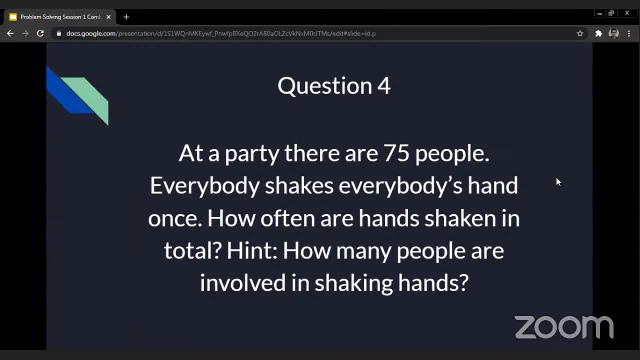 your logic is correct and your answer is also correct, and we can. we can think of it in terms of combinations as well, if no one else has any other answers, and i guess many of you got the right answer- yeah, it's seven. okay, okay, okay, i won't do it. 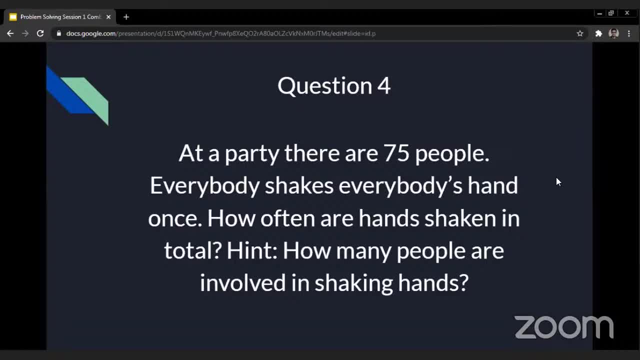 so many of you have got the right answer. and uh, this is indeed uh, and uh, actually uh, on hand shaking. there have been quite a lot of uh problems and uh, once in a while, these problems come out and they are not really simple. they are. so, again, this is a raw form. so this is even even this is a raw. 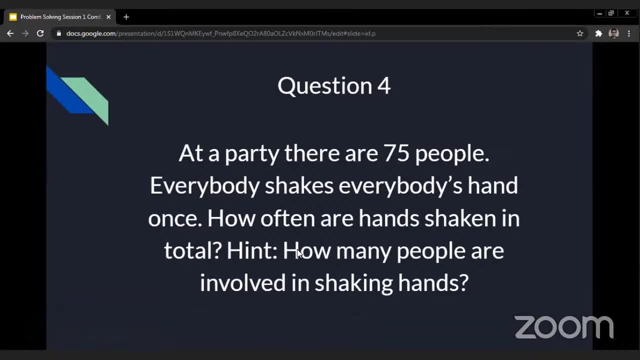 form of the questions that can appear in olympiad and uh, they're usually concealed. the most of them are hand shaking and there's even a lot of work on hand shaking. is a lot of work on hand shaking is a been there. there's a lot of theorems and lemmas in such such situations, such scenarios. 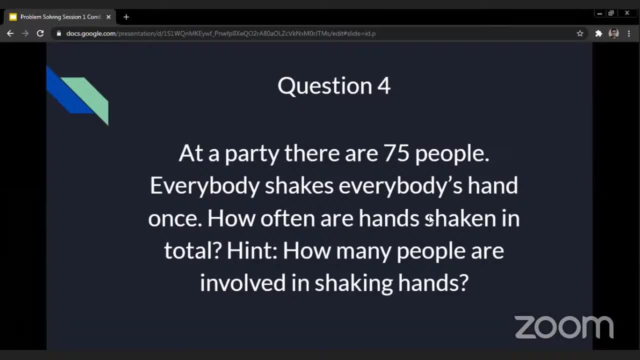 okay. so i guess we'll move on now to the solution. uh, just to make sure you all can hear me, right, okay, okay, thank you, thank you, okay, just to uh make sure, uh, now let's, uh, let's move on to the solution, and this is quite simple actually, uh, if you think about it. 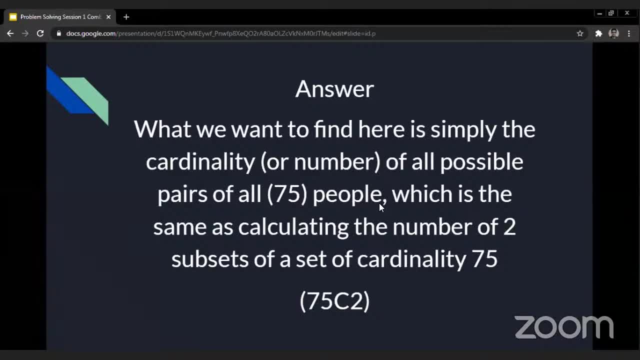 that all we want to have. when, when persons are shaking hands, we know that two people can shake hands at a time, and so, uh, it's not that every person will uh shake hand with the person with whom he has already shaken, and so we we rule that out, and it should be that two people shake. 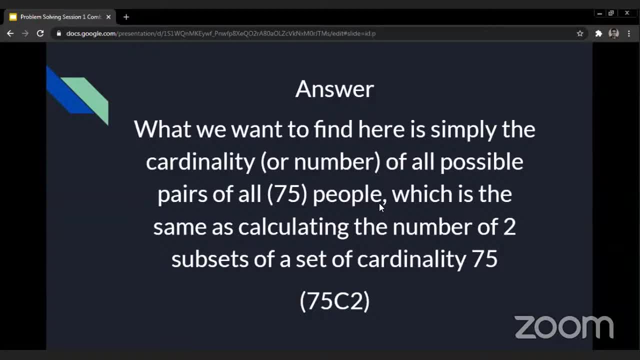 hands at a time. so you want to choose two people from 75 at a time. so that will be the number and that is 75. choose two, which i think is uh two, seven, seven, five, and you're right, uh, it's actually uh n into n minus one by two formula. so you can use that as well. you can use triangular number. 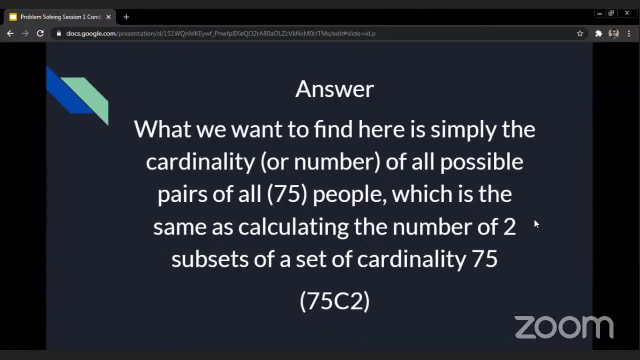 minus one there, okay, so, uh, i guess, uh, everything is fine here. if anyone has any doubt, you can put it in the chat, because, uh, i guess most of the doubts are resolved in there. yes, tanish, you can use that, right, okay, so i guess, no other doubts. then we can move on to the next question, which i think is a bit. 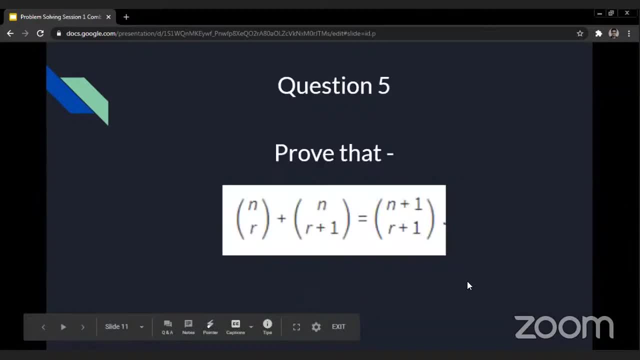 harder. let's see. okay, so this is a bit of an algebraic question actually. you can't put it in chat, but let's, let's give some time for people to think about it. don't put it out in the chat if if you get an answer, which is okay, well, actually, this, this question has two methods. i 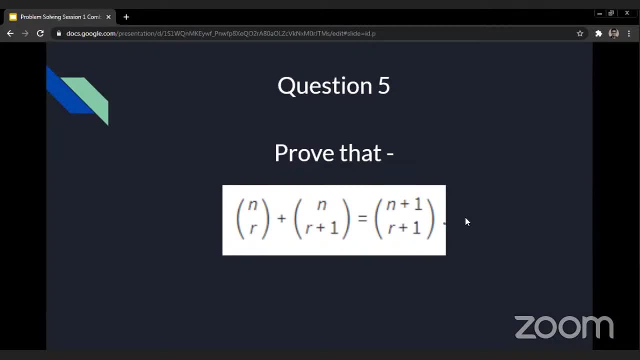 will be demonstrating you to solve, and the algebraic method is actually it's like you will be solving, but it's nothing. you just. you just have to equate both of the sides. you solve separately and you solve RHS separately, and you can. you can easily show both of them equal, but it's, that's not what. 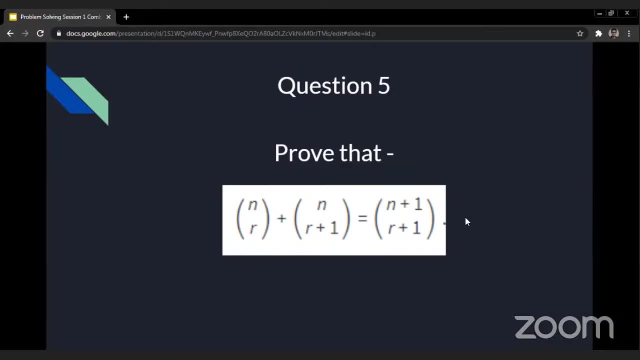 we want over here. what I want you to give you is an intuitive idea of why this works, so you all can verify this algebraically, and this is often called as Pascal's theorem, and you might guess where this is leading us to, and hopefully that is right. yeah. 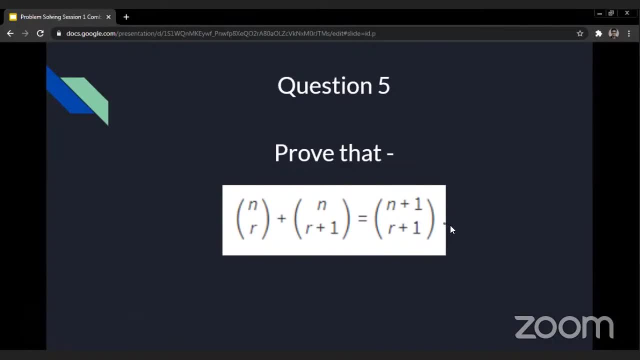 yes, Imran. and where does that lead us? to an extremely interesting topic and a structure which, which is quite fascinating. even I like it a lot. it's quite intriguing to me as well. okay, no, no, no need of multi-set permutations. we haven't even learned about that yet. 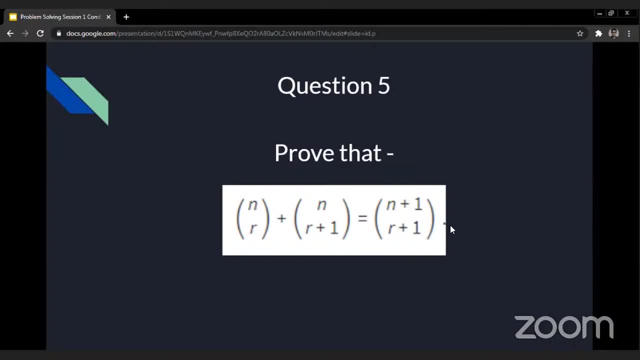 okay, we can do a combinatorial proof that way, but no need for that right now. I don't want you guys to be confused right now because, okay, Tanmay has got a non-algebraic proof. just just type out in the chat what the crux of your proof is, Tanmay, if you can. if you can just 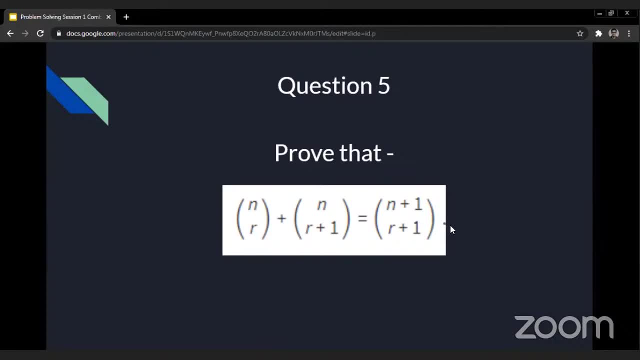 type out like one or two sentences of how you want. I guess. I guess if you, if you are thinking the same way as I am, then you might, you might be able to tell me in like three words, maybe two words actually. so, if, if, what, what is the crux of your proof? if you are, if you got a non-algebraic proof, then what? 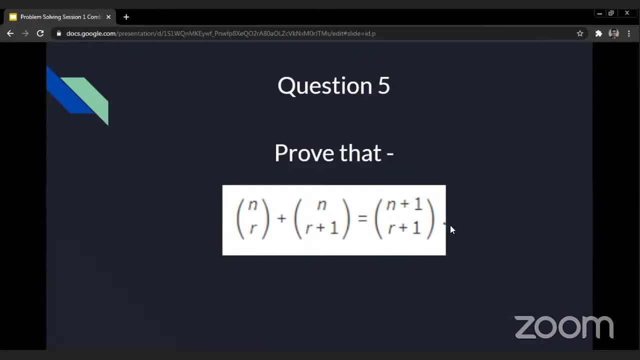 the crux of your proof is: okay, okay, okay. so I guess I guess this is a really nice place where I can ask Tanmay Sarada to just unmute and let's see what he has to tell us. okay, okay. so, after choosing r plus one objects out of n plus one objects, 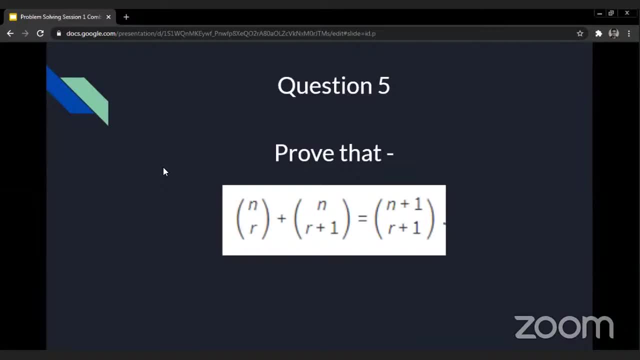 out of n objects, in the n plus one objects, there remains one object every time we choose it right. so actually, that is quite simply the crux of the proof, or the main idea is behind this, and this can be seen intuitively as well, but what i will be showing you is quite 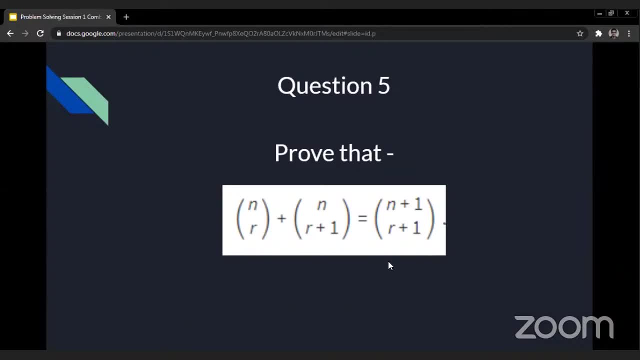 a different uh version of perspective, maybe, of of looking at this identity. this identity also comes quite handy uh in solving uh combination problems, because a lot of times in olympiad, uh you see, uh you're just given like 74 choose 3 plus 74 choose 4, and you can, you can simply substitute 74 if 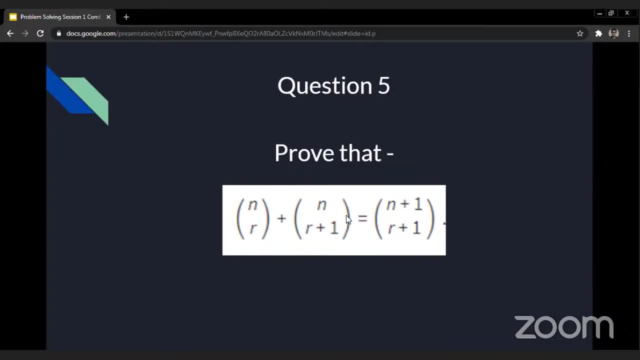 choose uh 4 for that and so on. so it's like one of those basic algebraic identities like a square minus b square or maybe something like that. uh, for those who have not verified this yet, you can all verify this algebraically and we have already seen why why this works. but i'll show you a different. 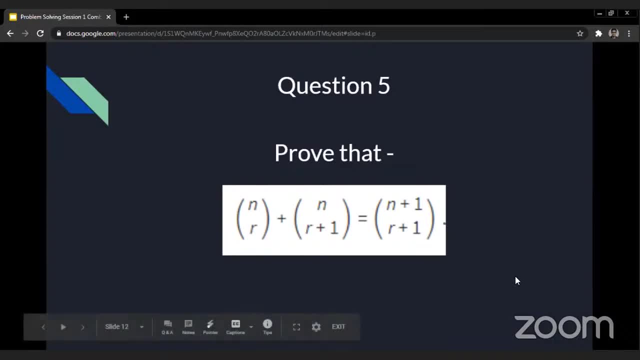 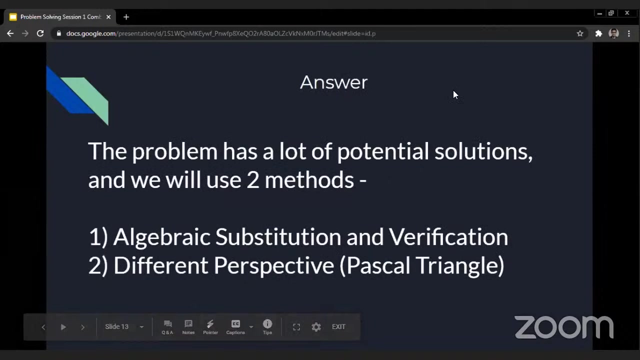 perspective of why this works. so, oh no, i'm not speaking right now, okay, uh, i was just waiting for a minute. okay, now let's, let's move on to what i have in for you, okay? so, uh, let's, let's move on. as i said earlier, this problem has a lot of potential solutions. 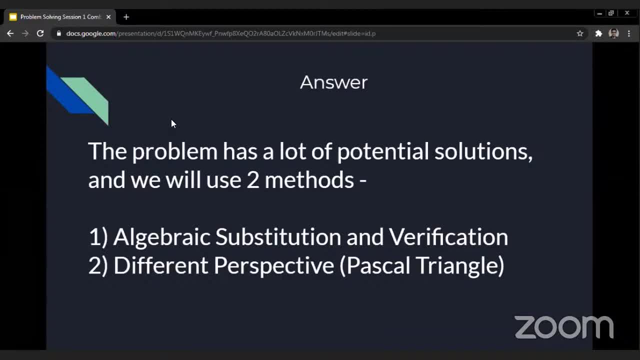 uh, one of them was: uh what uh tanmay told us, and what we we will be seeing is we used algebraic verification- and i trust all of you that you are great in algebra- and we have simply defined some formulas and you all can verify this really easily. but what i wanted to show you, uh what? 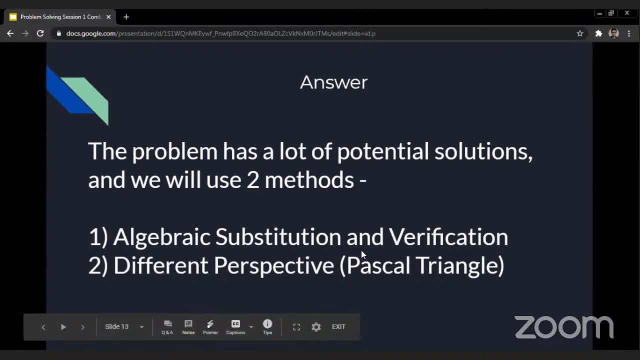 how beautiful combinatorics can be is uh, by having uh so many fingernails and using in this form. but here we have a Dah Yosh thisvell problem. sticks like so, but there's a very difficult problem not to confuse with any Galically. so let's, so, let's start off with analysis. what is the galically? 1 n 귀ных times. 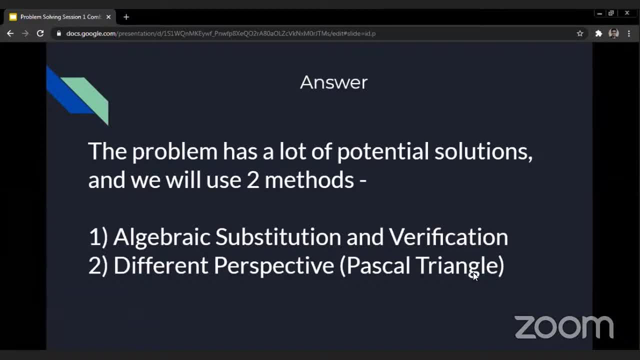 surveying. so, um, eventually, combinatorics, or it's a part of some other areas in math as well. it comes up when you are studying the binomial theorem as well, which will be studying. the next topic will be studying in combinatorics, and that is quite handy. it's a beautiful piece and it actually to be precise. 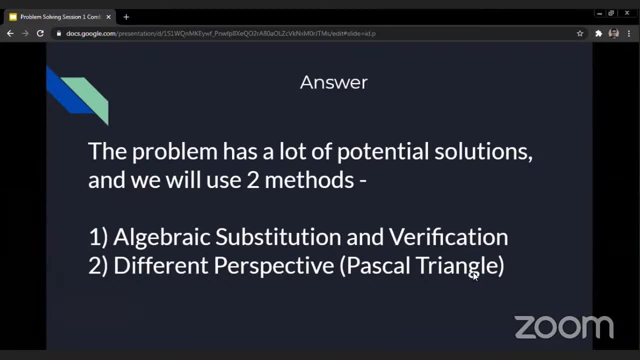 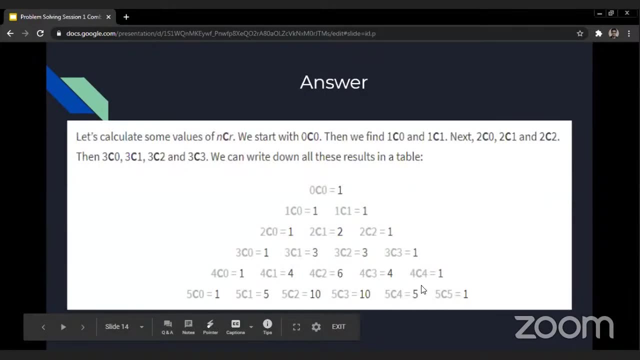 it was first first given by an Indian mathematician called Pingala, and what Pascal has done is a slightly abridged version of it. so let's have a look at it. so this is the Pascal's triangle. you can ignore these grace, grace numbers and names for a while, but what? what I want you to? 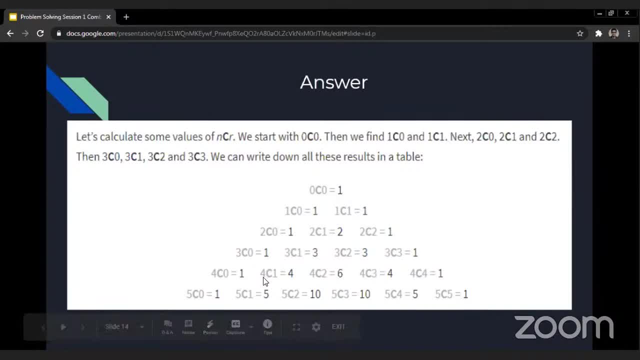 see for the first time is this: just see and make some observations, like you can have observations like the first row is one, one, one, one, one, the second row is one, one, one. I mean, this diagonal is one, this diagonal is one. then if you look closely, then this, this diagonal, is one, two, three, four, five, that's all the natural. 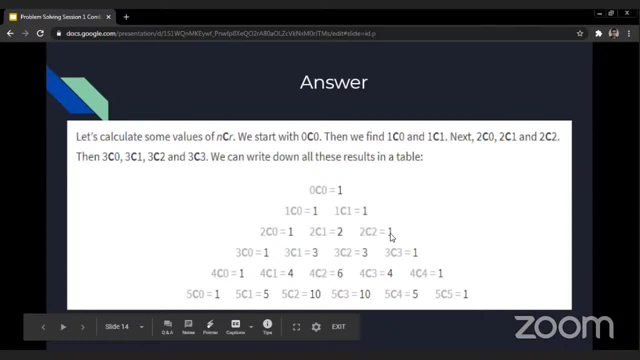 numbers, and if you look even closely, then this diagonal is one, three, six, ten, which is, I guess many of you know as the triangular numbers, then and so on. we have a lot of patterns in this. even the Fibonacci sequence comes up in this and I don't want to go into that. but how do we define this? so if we calculate some, 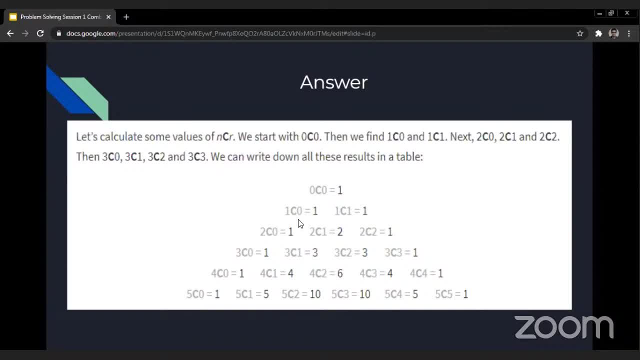 values of NCR. we get 0- choose 0 is 1. then we have 1- choose 0 is 1, 1, choose 1 is 1. then we reconstruct it this way. and if you observe neatly, if, if I were to, if I were to tell you at first and I gave you 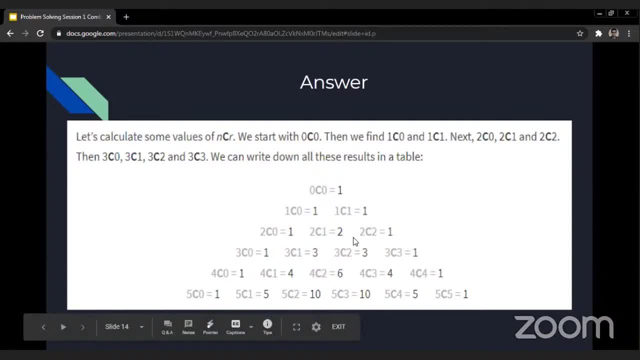 this part of the triangle. you would be able to complete it by seeing this pattern, that is, one plus two, three, two plus one, three, three plus one, four, three plus three, six, three plus one, four. and this one is here: one plus four, five, four plus six, ten, six plus four, ten, four plus one, five, and this way: 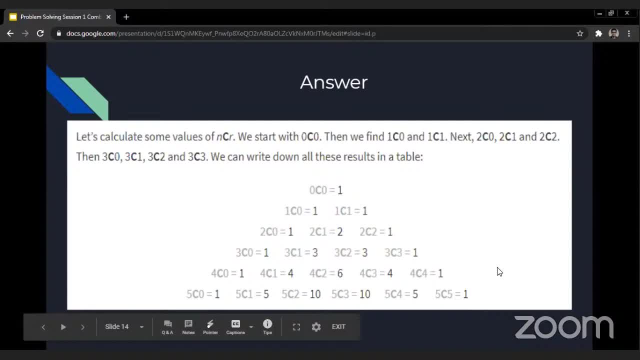 you can easily complete the triangle. but what? what are we doing if you, if you just have a look at it, we are doing four, choose three plus four. choose four is five, choose four. and what? what's our identity saying, what's our identity asking us to do we want? 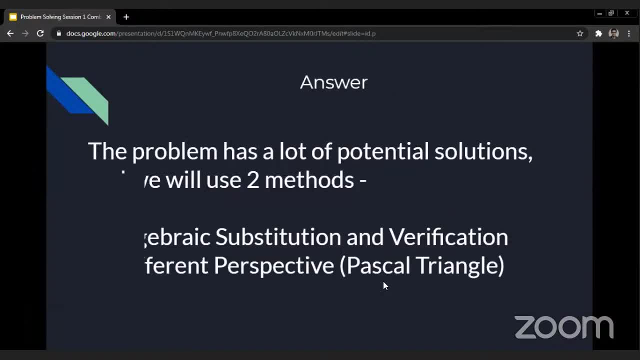 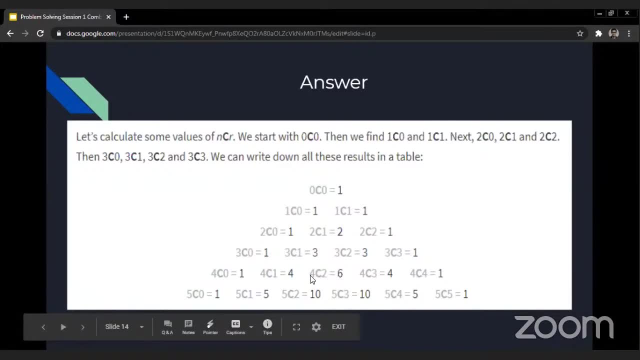 to prove that n choose r plus n. choose r plus one is n plus one. choose r plus one. and that's exactly what we are observing here. like uh, you see, if n is four and r is two, we have n choose r plus n. choose r plus one is n plus one. choose r plus one. right, isn't this right? 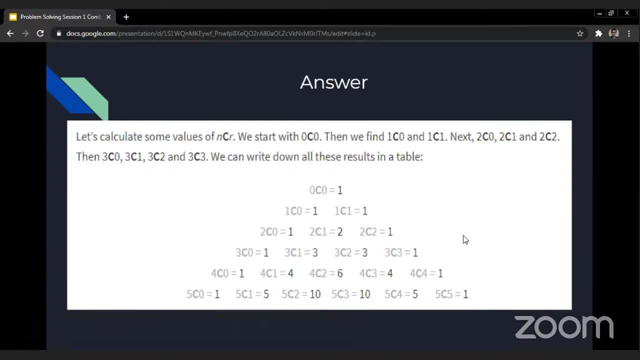 so this is a different perspective of why this works. we can even uh maybe get a combinatorial proof or something like that, but uh, it's not. this is, this is the beauty of uh combinatorics, as I uh, I would uh say it. but this this is also linked to the binomial theorem, in the sense that uh, in the 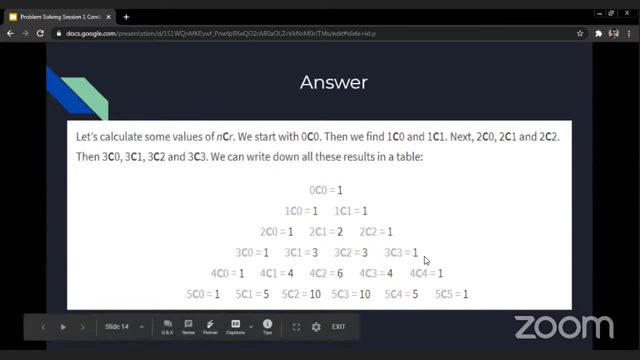 binomial theorem. uh, if some of you may be knowing that, uh, the Pascal's triangle gives us the values of uh, x plus y raised to the power of n and y of n plus one. and that's exactly what is happening here. to n uses the coefficients of all the, of all the variables in x plus y raise to n. but we will talk. 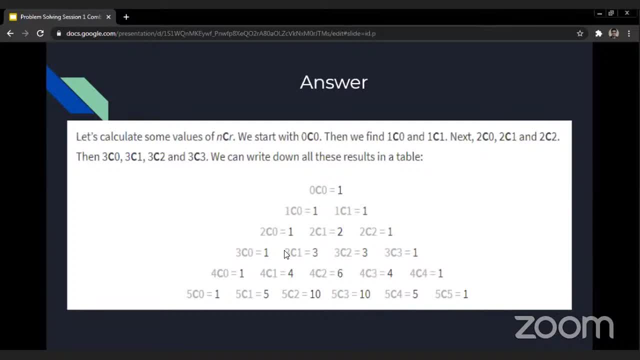 about that later, because right now, i want to focus on this perspective of it. so i hope all of you see this pattern and this is just simply. this is an observation, okay, and it's it's a way we constructed it that makes it happen this way. so if, if you, you go on and tell me that what you have shown me is 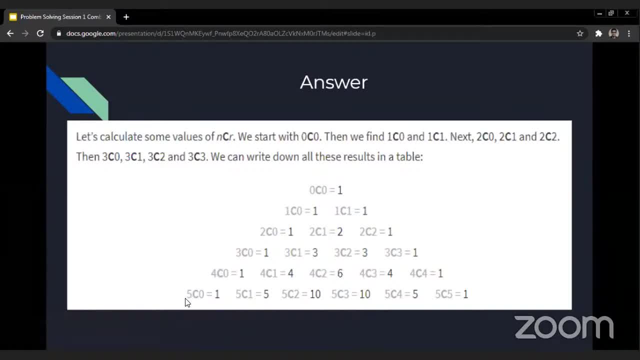 just an example. i would say: no, this is a proof by construction, and that would also be a different proof method to be talked about later on. but i'll just give a glimpse. so if we construct something and we construct it in a specific way, suppose we have a construction like we- we constructed our. 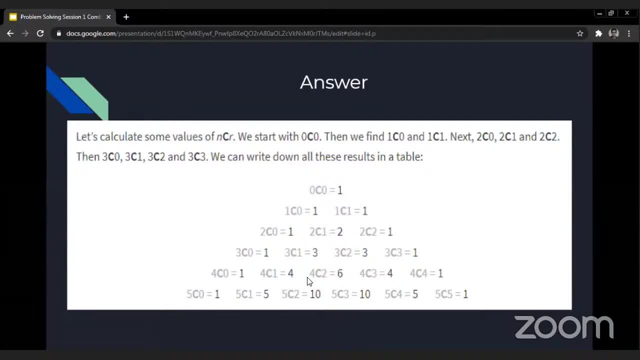 scenarios. we constructed our examples and we constructed it using variables in a specific way so that one or two of theorems or observations always happen. then we can prove it using construction, so we can say that it is proved by construction. and this usually occurs in discrete math- a lot, but i don't want to talk about much right now. 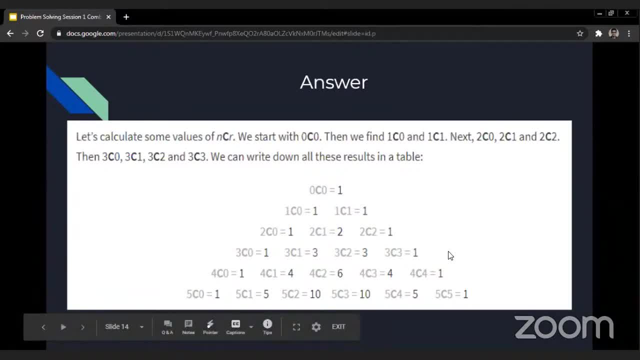 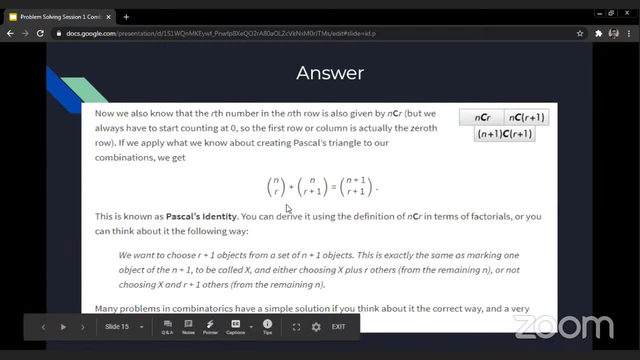 so i hope all of you can see how this works out, and this is just writing it down formally and you can all read this up. this is the pascal's identity and this is what tanmay sarda told us. we want to choose r plus one objects from a set of n plus one objects. we begin with the right hand. 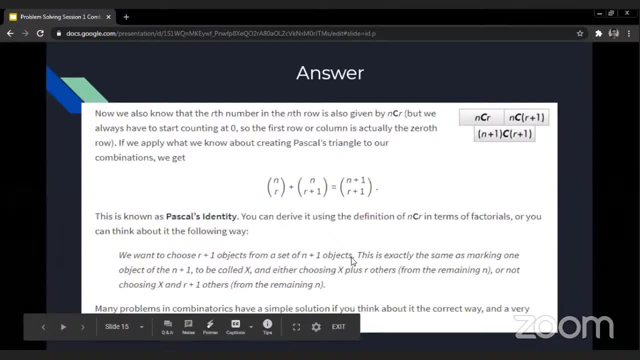 side. okay, i want to choose r plus one objects from a set of n plus one objects, and this is exactly what we want to do. we take an object and we mark it and let it be x, and we either do x plus r other from the remaining n or not choosing x and r plus one others from the remaining n. and this is, this is. 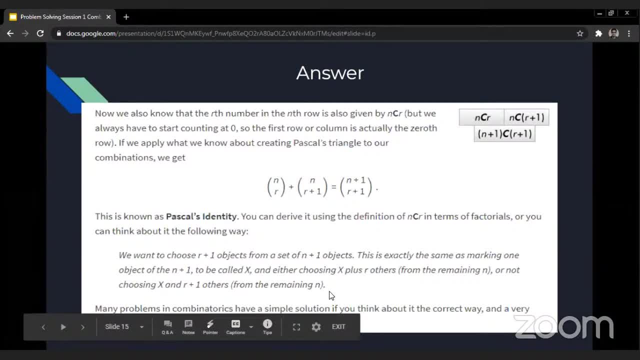 uh, like you can. you can think about it as you are taking x, but you have r others left, so you you take the r others, uh differently, or you don't choose x and you take the r plus one others differently from the remaining n, and this is exactly what we want to do. so we take an object. 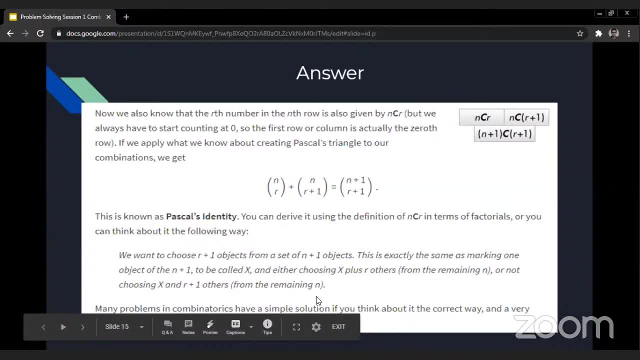 the remaining n. both of these times you have n n. so here you are choosing r plus 1 and here r, so what you get is n choose r plus n. choose r plus 1 is equal to n plus 1. choose r plus 1 and. 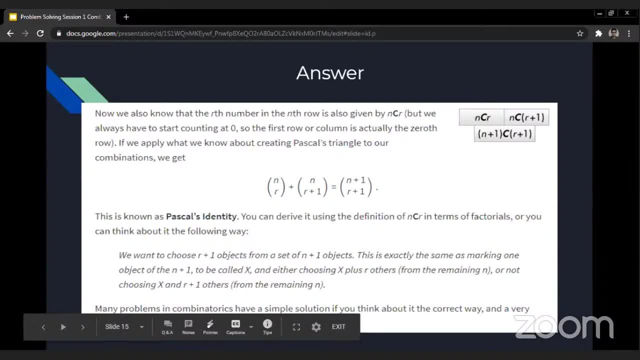 that is a logical evaluation of this thing, so you can just, uh, have a look at this and if, if any of you don't understand this, just raise your hand, because i think this, this is quite understandable. i hope all of you understand this. thanks, thanks, okay, uh, how many of you feel that this is really beautiful? because i think that 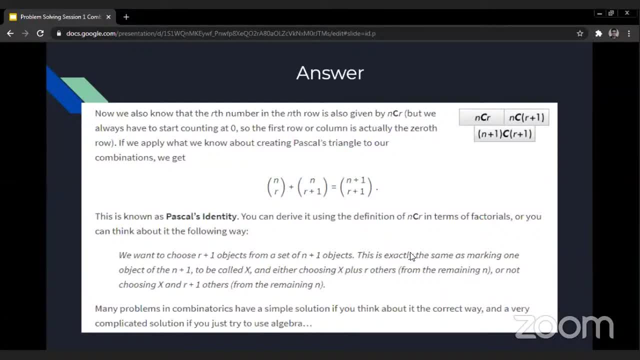 this is one of the- uh. this is some uh. what we are exploring right now is a really interesting field. it's, uh, the. the interesting thing about this is not that it it is beautiful or something like that, but the thing is how we can correlate different areas in mathematics, and half of the areas that we will study in mathematics are 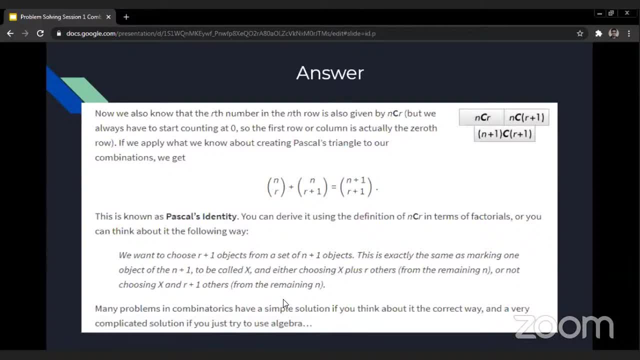 correlated like this. in this way itself, they turn up everywhere like, uh, yeah, yeah, right, right, oh no, let it be, let it be imran, that's. that would be a bad comparison. actually, great, uh, although, although, uh, it's not that, um, all of you must feel that it is interesting. i. 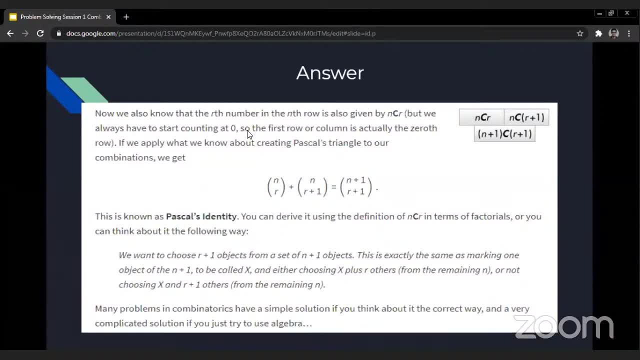 just i just uh told you uh what, what my perspective of it is. because uh having something taught to you in this perspective makes it feel much, much better than what you think it is. because uh having something taught to you in this perspective makes it feel much better than what you think it is. because uh having something taught to you in this 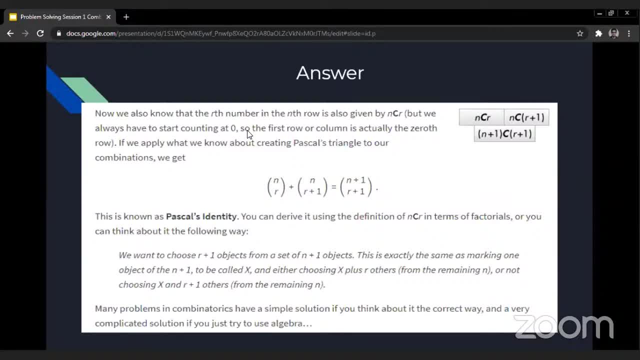 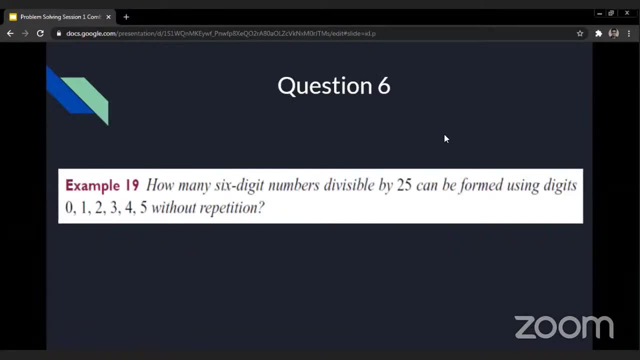 more interesting than you just explaining uh why- why this works. so let's move on to the next question, as we are running out of time and i'll just give three minutes to solve this. and, uh, to be frank, i have taken this uh out from a book and i can share this with you later on. 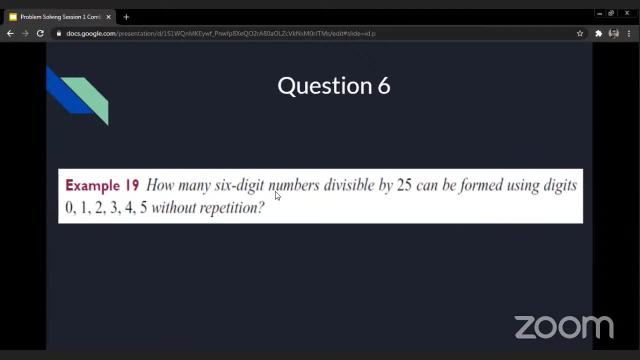 but this, this is one of the most basic problems and such problems. i now i'm uh, this, this is not a really basic problem actually, uh, but the thing is that such problems- this is the. this is an example of a coated problem. it's not raw, so this uses. 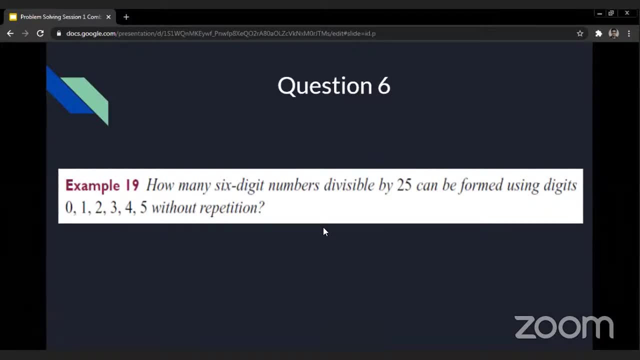 multiplication principle and, uh, if you want, you can use combinatorics, but i don't suggest using combinatorics. you can, you can do everything using multiplication principle, because whatever we have looked at has been done by multiplication principle. whatever you can do using combinations and permutations, you can definitely have a solution for it using multiplication principle. 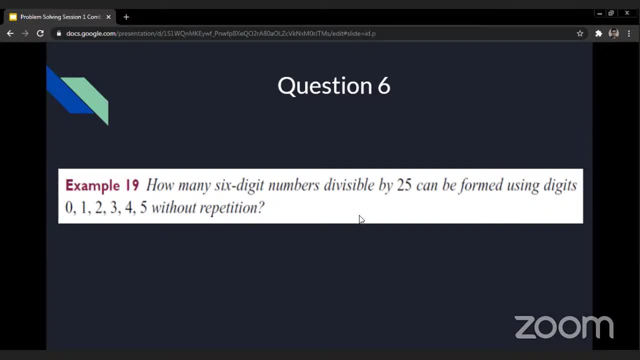 multiplication principle. all right, yeah, that that would be a a great way, and i'll give you out a hint, and that is what tanmay sarda has told me- that, uh, the hint will be that, uh, look at this, divisible by 25. okay, so you have. 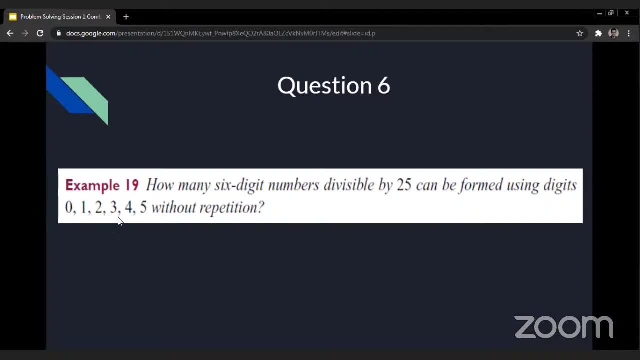 you have, uh, these, uh these digits, one, zero, one, two, three, four and five, okay, and uh, you don't. you cannot use repetition, just just have a look at it neatly, because sometimes you get confused just because you don't look at the question neatly. sure, sure i'm, i'm waiting for some time, uh, 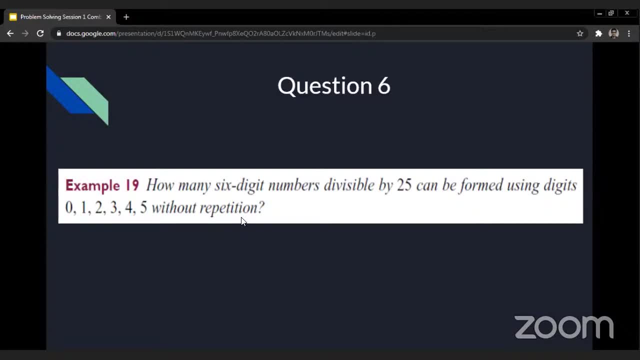 that's perfect, samyak, perfect, really elaborate, and i like the way you uh told me. uh, imran, i guess that is wrong. i don't think that is right. you can, you can think of it, uh, some more time. the hint is that you can take two cases. 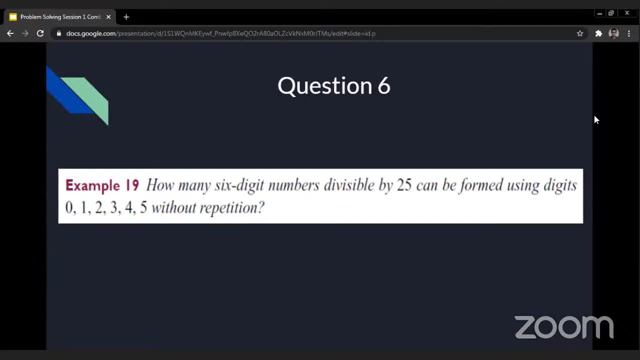 consider two cases. yeah, that's what happens most of the times. whenever you see such a thing, you, you, you can go about it using cases, but that becomes much more useful than using and doing it together. so it's easy to use cases and it just sorts things out perfectly. right, finish, that's right. yes, right, Imran, got it this time. oh, I sent me. 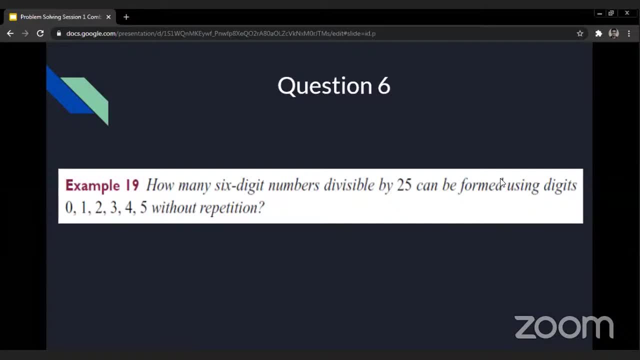 this. okay, then my 18 is not right. you must, you must think it's actually one part it's. it's one case. I guess I think so. it's one case. I am not really sure, but I think it's one case of I want you to think it's not big, it's really small, it's less than 50 to be really. 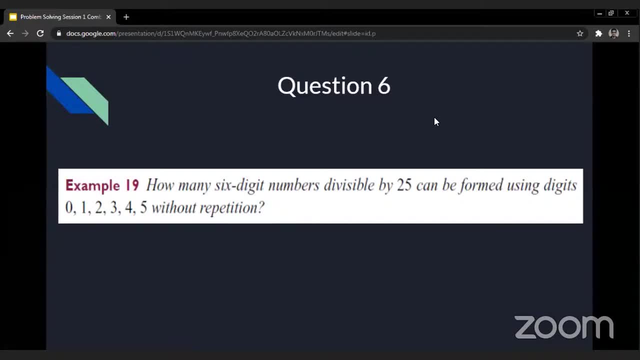 uh, what can I say? yes, yes, Imran, okay, okay, uh, yeah, I still want others to participate in the discussion. I've, I'm, it's not a discussion, actually, it's a one way. oh, am I? only I am getting all the answers. so, uh, but uh, uh, others can definitely uh text their answers to. 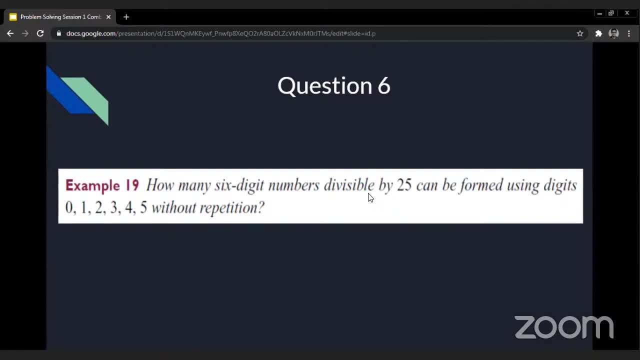 me whether they should be right or not. I am not asking you to give me the right answer. yes, yes, Imran, right, right, Tanmay, now you got it. the second case, see, it's uh, it's a different thing to be solving such problems and, uh, they are not really simple. I agree that they are not simple. 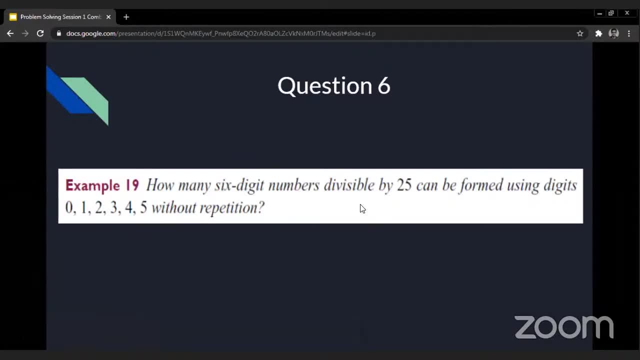 but I don't want to be solving such problems. I don't want to be solving such problems. I want you to give me the right answer as well. right, I want you to try. just send me an answer why it should not be random, right? I don't want the random numbers to be sent out to me. what I want you 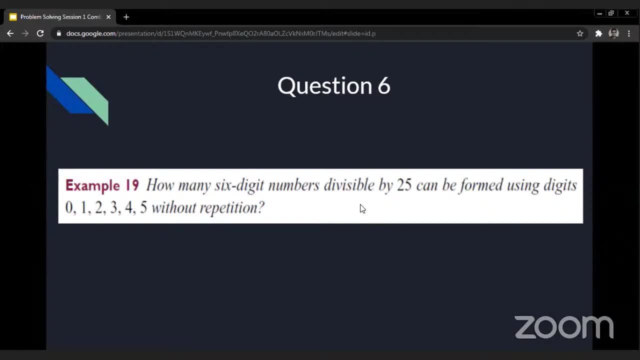 all to do is to try to solve these problems and if, if you get an answer, you can send it to me. I can verify it. if it's not right, then I can tell you why it's not right, because, uh, you don't get this experience again, you, you, you will be able to solve problems only if you solve a lot of problems, I mean. 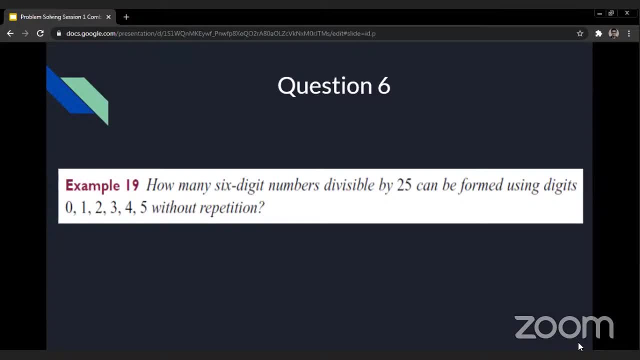 you will be able to attempt Olympiad problems only if you have experience of such problems. this is really necessary for uh being able to score a higher score. what, what uh? this is an example of uh problem solving ability. it's uh, it's purely your thinking skills that come into play here. 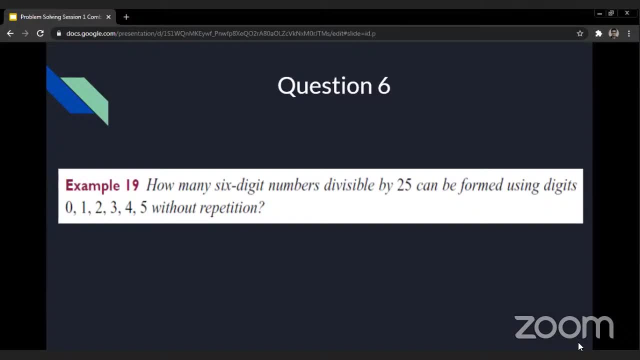 even if your knowledge is limited, then you can. you can attempt such problem solving schools which are development teachers to attempt these kind of problems in your sentence. uh, all right. so I think we colleges today can already tell if we don't break any rules, because we see what's faced us when we are downloading. 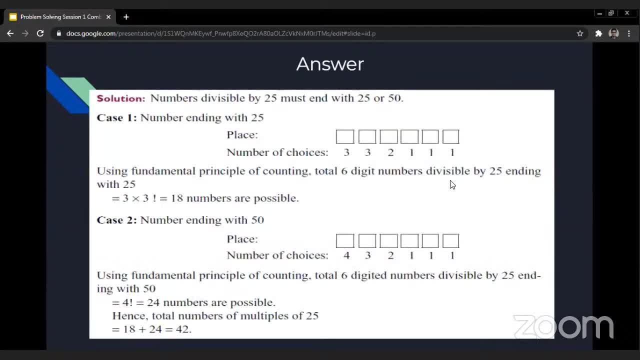 uh, 직접 learning atheism play scenes, or we can learn how used to reading. here's our 2nd statement. Yeah, it's right, Archit. Yeah, I've got a lot of answers now and most of them are correct in camp, and so you just, you just check how many choices are possible for each. 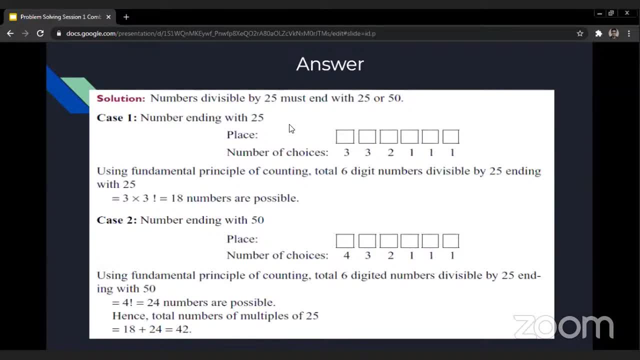 place and then you just find the number, number of possible choices and just add them up. so this, this comes arbitrarily due to the given things, because we are given whatever we are given we can use these things for, for these choices, and they influence the choices completely. so we are using multiplication principle. 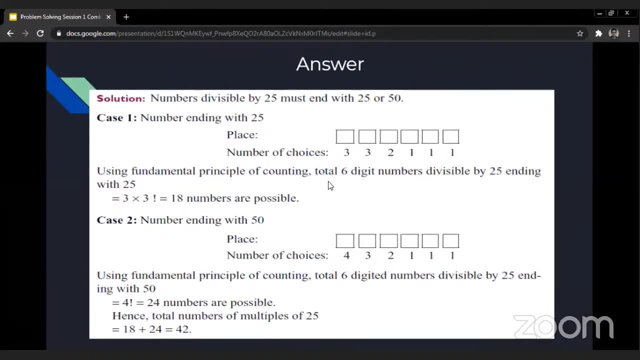 here it's written as fundamental principle of counting over here, and okay, so the second case: we still have four, three, two, one, one and one number of choices according to whatever we know as given, and that comes quite trivially because it's it's not too hard to. 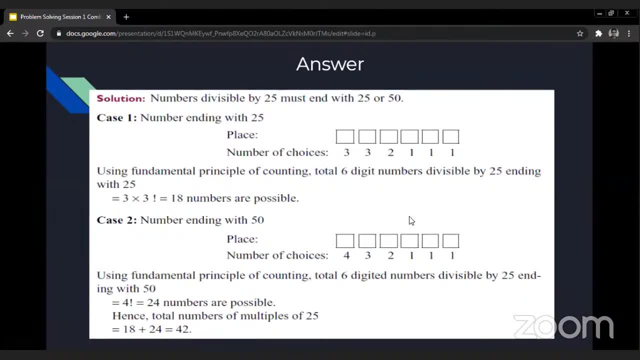 imagine that, and we have done that before, so the correct answer is 18 plus 24, which is 42. I hope everybody got this right. we are running low out of time, so I should be going on to the next question and I'll have to give only two. 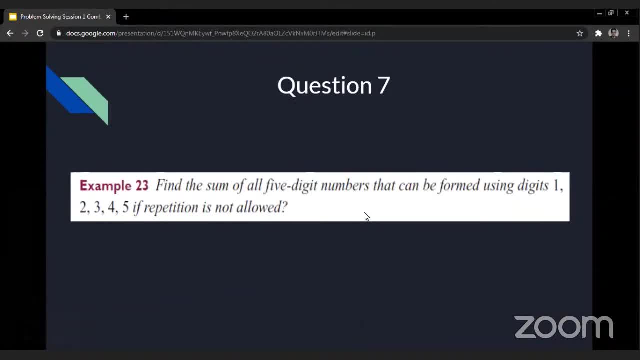 minutes for this question. well, this is a. this is quite a hard question. I don't expect all of you to get the right answer, but whatever answer you get, then you can just send me. yes, Imran is. this is a really nice problem actually, and here this is not like you cannot list out all the cases, because, oh, that would be that. 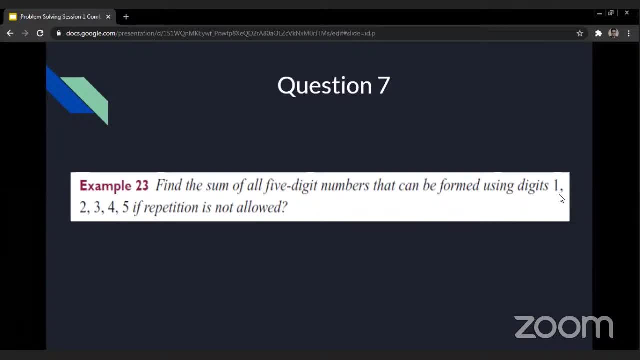 would be. that's five digit numbers and you cannot just list out all of the number six. well, I don't really know what the answer is, but I will have to wait for everyone to solve and then we'll move on to the solution, because the answer is quite big, according to what I know. 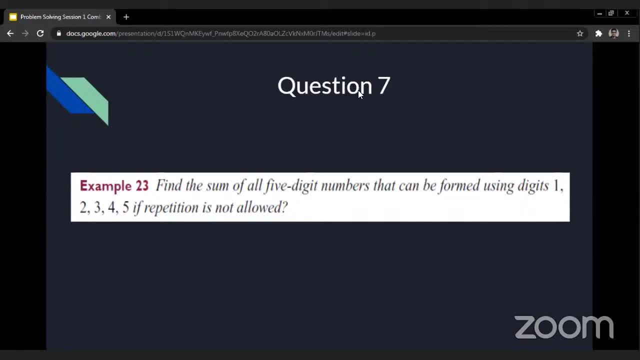 so I didn't memorize it. I'll have it on the next slide. only one or two more minutes, because we have really less time. we have around two more questions. so, guys, this session will have to be extended for some time. not a lot of time. I did 10 or 15 more minutes. 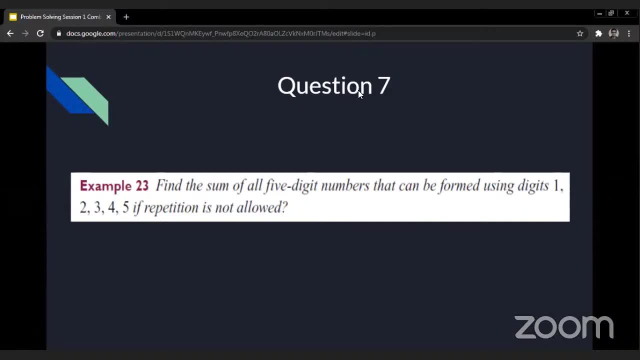 but I guess you are enjoying, hope you are enjoying last one minute for this question now, because we are going to move on to the next question and then we'll move on to the next question and then we'll move on to the next question. so, guys, this session will have to be extended for some time- not a lot of time. 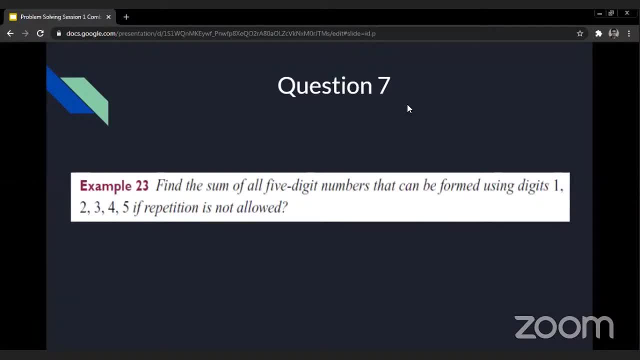 but I guess you are enjoying last one minute for this question and then we'll move on to the next question. so, guys, this session will have to be extended for some time. not a lot of time, but I guess you are enjoying last one minute for this question and then we'll move on to the next question. 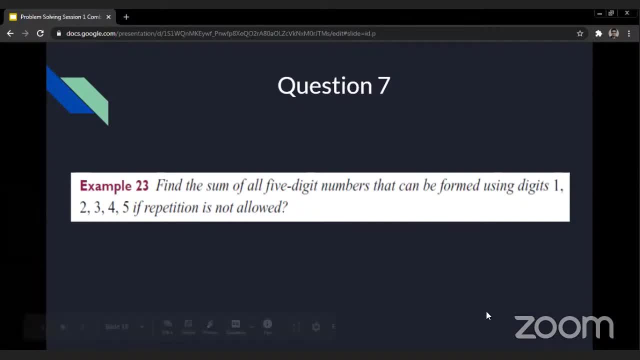 so, guys, this session will have to be extended for some time. not a lot of time, but I guess you are enjoying last one minute for this question and then we'll move on to the next question. so, guys, this session will have to be extended for some time- not a lot of time. 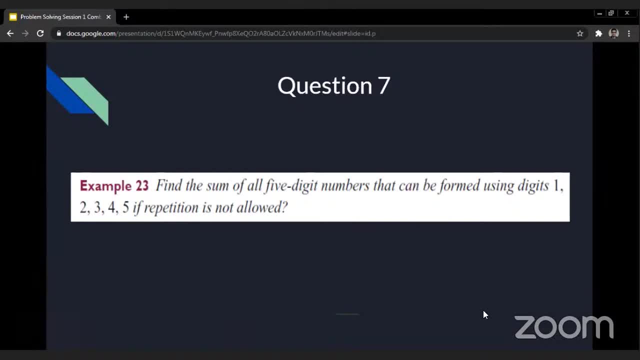 but I guess you are enjoying last one minute for this question and then we'll move on to the next question. so, guys, this session will have to be extended for some time. not a lot of time, but I guess you are enjoying last one minute for this question and then we'll move on to the next question. 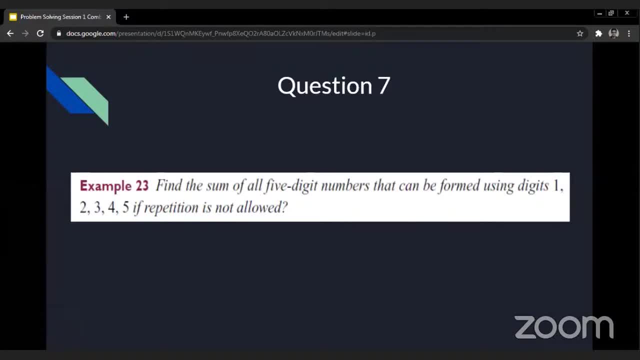 At least they seem to be the same Right, Samyak, That's the right reasoning that you can use And this: we will be using a different perspective to solve this problem. We don't have a lot of time for that, Imran. 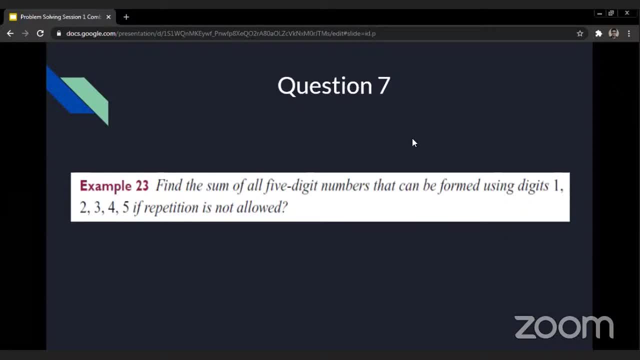 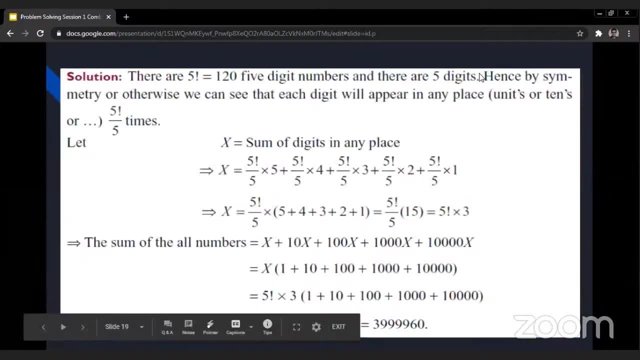 So I don't think that would be a good idea, because we are already running out of time. I still have two questions, I think, to go. Let's move on to the solution now. I guess a lot of you have given me this solution, which is right. 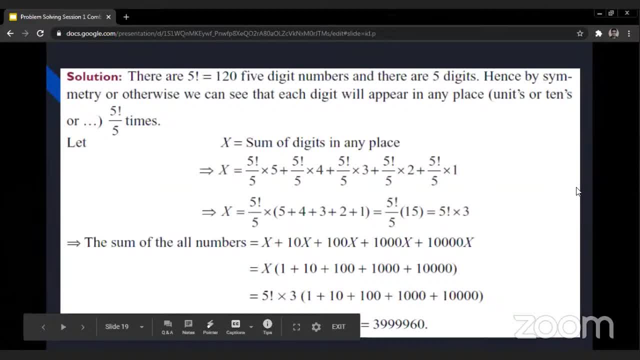 Tanmay, what solution did you send me? 15 times 4, factorial times 1, 1, 1. 15 times 4 factorial is the same as 1. 20 times 3, or what? No, I don't think. 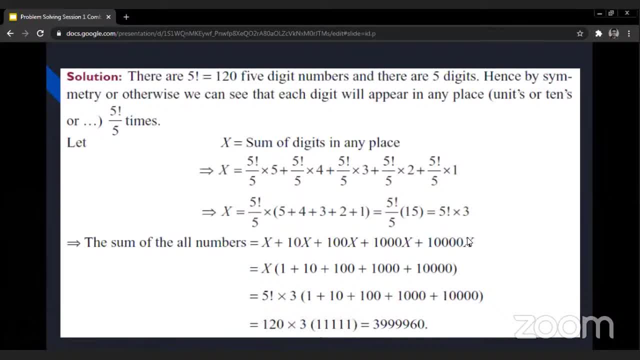 There's a slight modification in your answer, Tanmay. Okay okay, okay, okay, Okay okay. So what we do here is that we, instead of we, again partition the problem, So we don't want to solve the same problem, because that becomes quite tough. 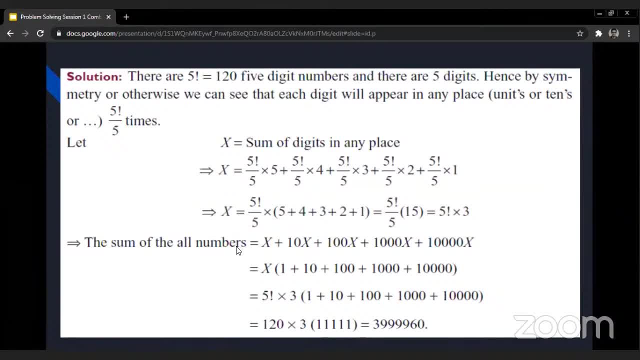 So what we do is we partition, So we partition the problem somehow. and how do we partition the problem? So, first of all, note that there are 5 factorial total amount of permutations that are possible, And we have 5 digits. 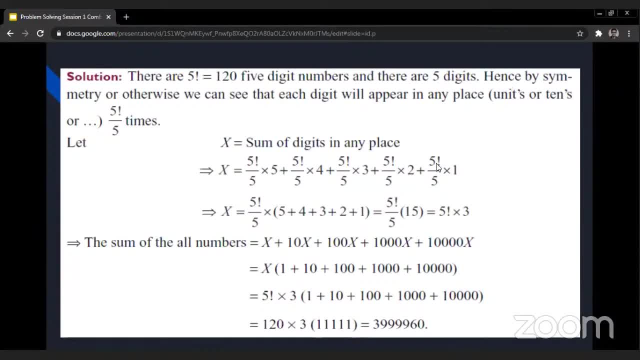 And if we looked at it using a tree diagram? ignore the symmetry because we haven't learned about it, But if we were using a tree diagram, we could have easily told that this: each digit appears in a place 4 factorial times, with 5 factorial divided by 5 times. 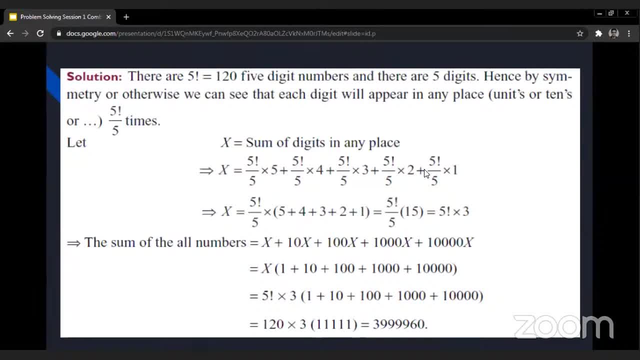 So, instead of doing it this way, in the normal way, what we do is that we just take a variable, x, that which denotes the sum of the digits at any place, And so, instead of taking x as what we exactly want, we do something that is easier. 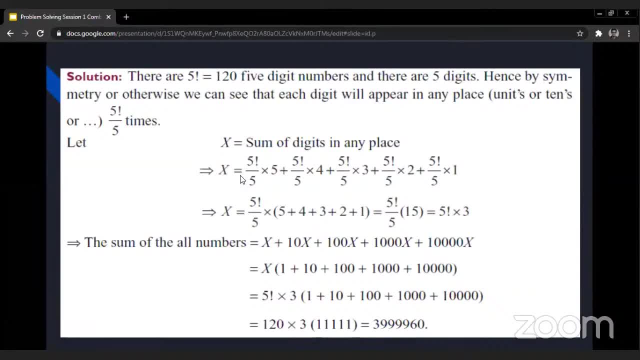 So what the sum comes out to be is x, which is 5 factorial divided, 5 factorial divided by 5 times 5, and 5 factorial by 5 times 4, and times 3 times 2 times 1, and we are using a 1,, 2,, 3,, 4, 5, right. 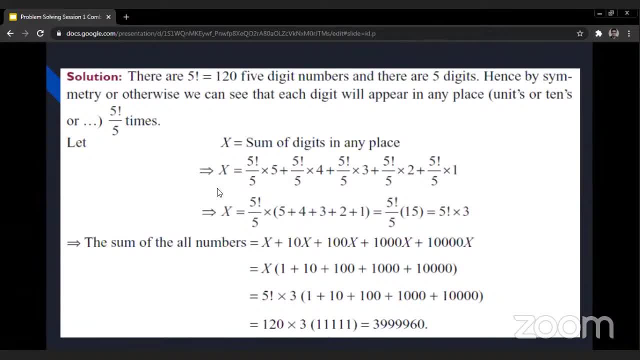 So what we get is this: 5 factorial by 5 times 5 plus 4 plus 3 plus 2 plus 1, which is 3 times 5 factorial. And now what we want is the sum of all such x, because this represents 1 digit. 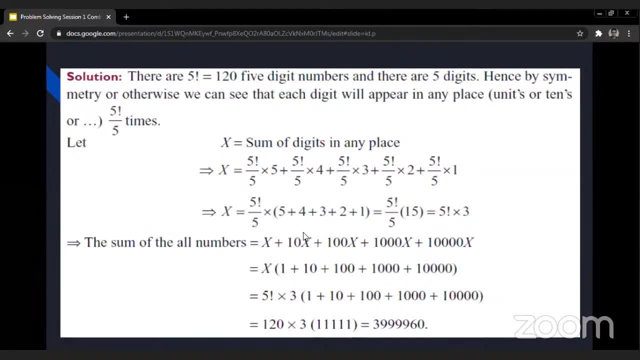 And we want A 5 digit number. I guess, Yeah. So what we want is would be 10,000 x plus 1,000 x plus 100 x plus 10 x plus 6.. And that is the same as 5 times 1 plus 5 times 1 times 3 times 5 factorial, which comes out to be this huge number, that is, 3, 9, 9, 9, 9, 6, 0. 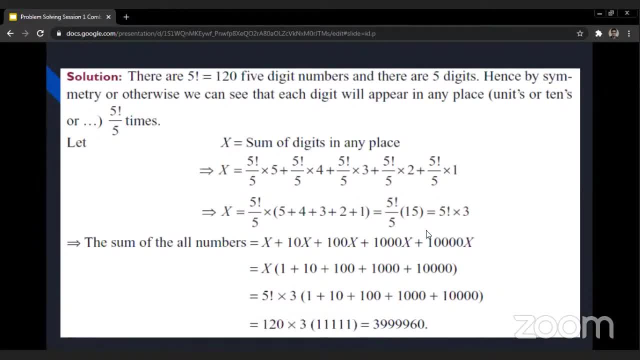 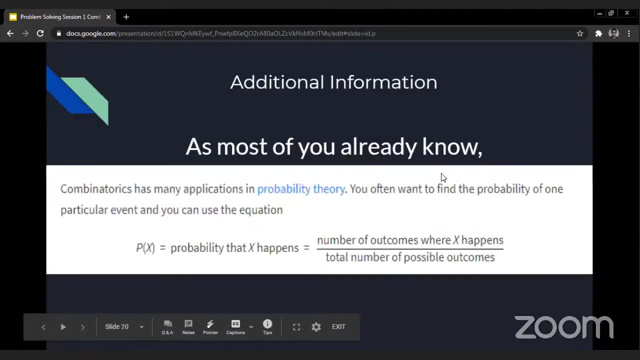 Okay, Tanmay, that's the same, And then well, it's really nice. So I hope all of you appreciate this thing, because this is a different perspective of solving, yet another perspective of solving such problems, And let's move on. 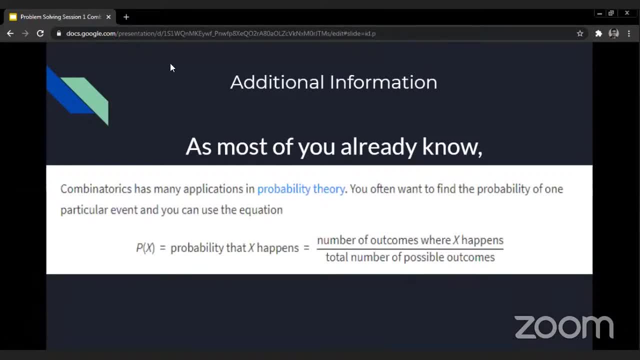 So this thing is really for a simple problem. I just want to make sure all of you know about this. So probability that x happens is just the number of outcomes where x happens divided by total number of possible outcomes. The question based is: 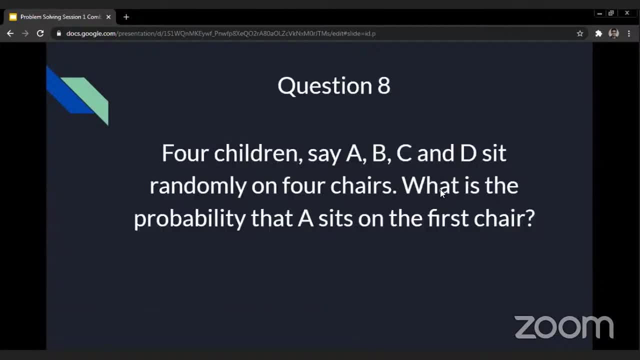 Is the number of possible outcomes that x has the overall probability that x has the overall probability that x has. And we have four children. Even we can do without their names, but they are sitting randomly on four chairs. What is the possibility that a sits on the first chair? 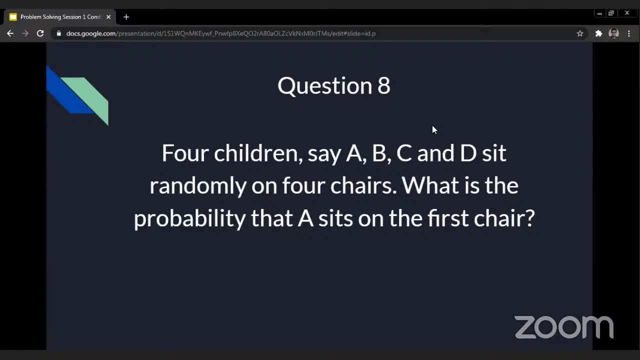 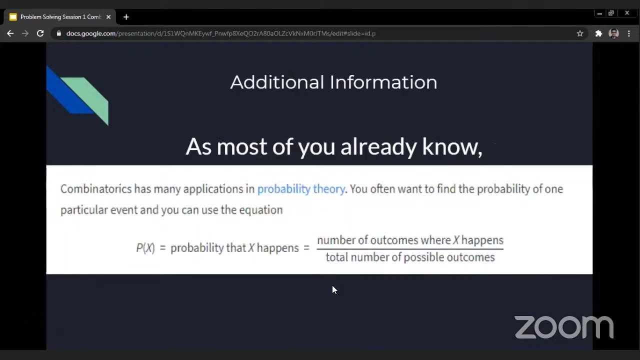 Just type out the answers in the chat to me, And it's really simple Actually. if you think about it, You can go in any way. It's. it's quite simple. if you know this fact, then it will be quite simple. Imran, I think you. 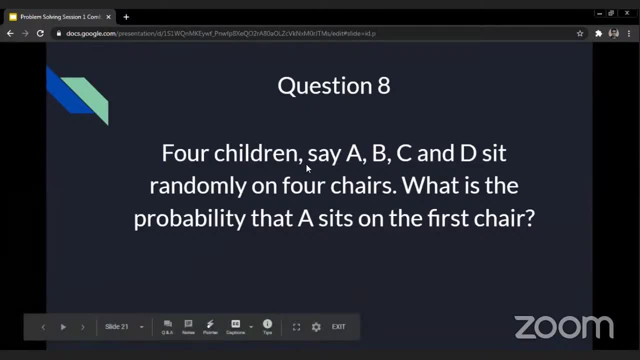 misunderstood the question, because it's not 1 by 4 factorial right now you get, okay, okay, well, using exclamatory symbol sometimes becomes quite tiresome if you are using for factorial as well, right, right, a lot of people have given me the right answer and which is really correct, and it's quite easy. 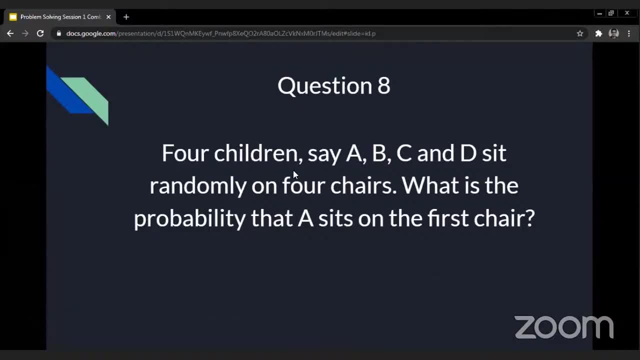 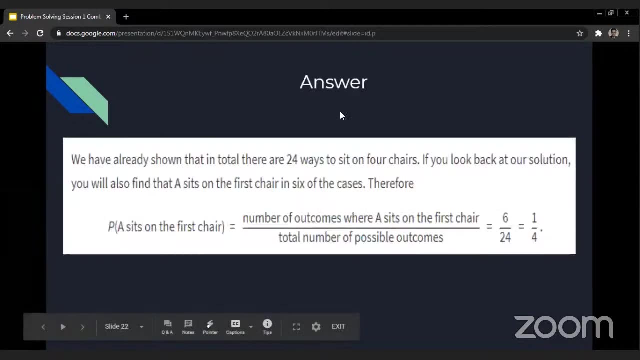 I think that is right, something that is right. that is right. Imran is right, Tanmay is right. okay, Tanmay got it using two methods. Tanishq, that is right. Aditya, that is right, okay, so the solution is this: what can we use? okay, okay, no need of combinatorics, right? so actually a. 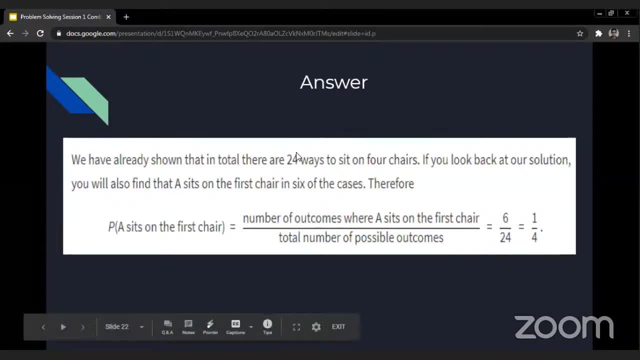 probability and combinatorics are really special bond, because a lot of times you can see combinatorics as a special bond, because you can see combinatorics as a combination of two different things. yes, so that's how we get it: the common combinatorics being used in probability to find the cardinality. because in 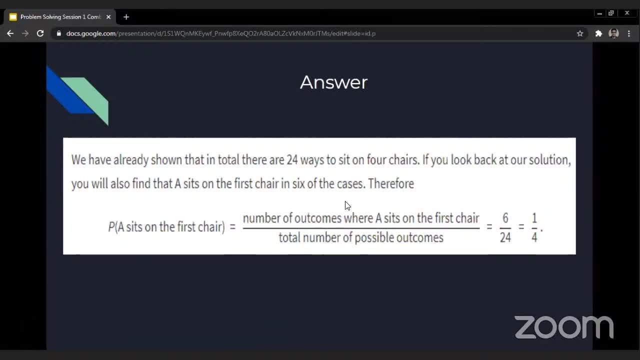 probability. we want to find the cardinality, because we need the total number of possible outcomes, and that is a cardinality, and this is a cardinality as well. so this is how we get 1 over 4. you can ignore this part, it's just this. 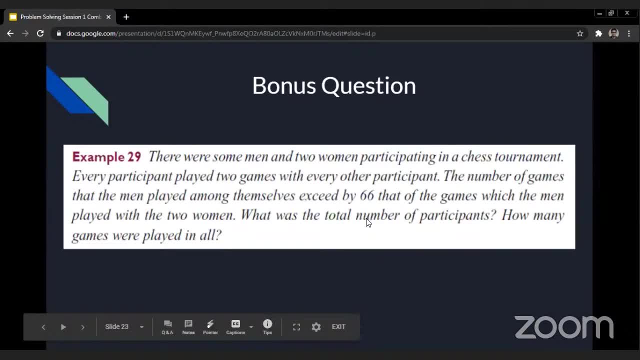 that matters- and this is a bonus question, right? this is quite tough, so let's see if we can just tough. those who have any other assignment or classes can leave, if, if, if you are free, then please stay and you can try this question, because this is a. 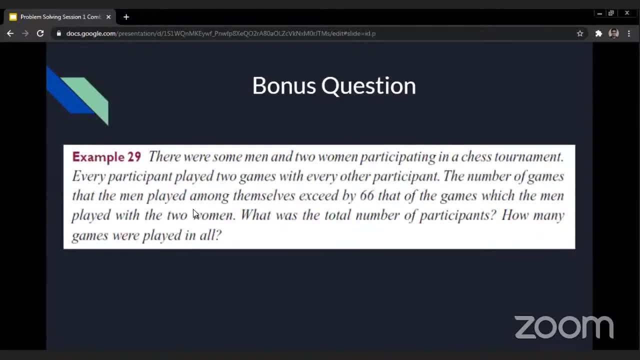 really fun question, actually, and it's a practical usage of whatever we have learned about combinatorics. if you look at it closely, then what this game tells you is that there are some men and two men participating in a chess tournament. so this tournament questions come up really really a lot of times in 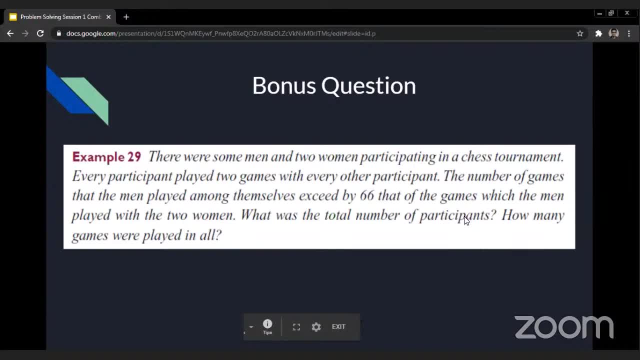 combinatorics and in probability and there are a trademark of such questions and they often come up in NMTC, in PRMO and even in RMO level examinations. we have such question like in probability. a lot of questions of the chessboard are quite stereotyped and just like that, some questions of tournaments are quite 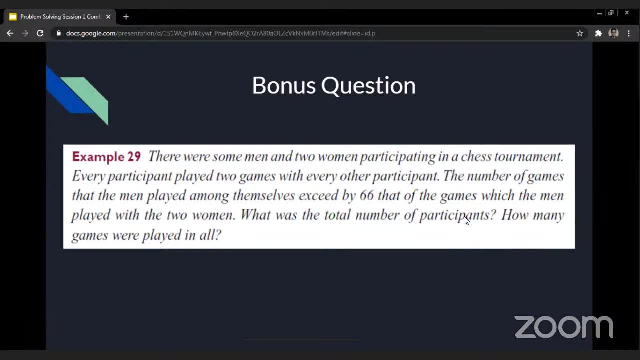 stereotyped in in combinatorics as, as some you know, I mean as a level problems, they are compared to as level problems. I don't, I really don't know the answer of this. I'll have to see some other questions. but anyway, going on there, we have another comment. 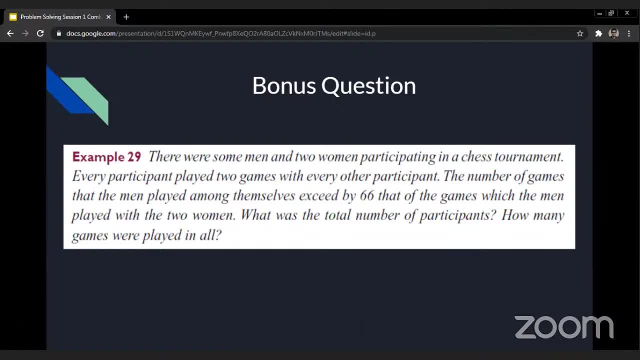 ok, someone is applying to the생방지com. ok, so what we are asked is: what was the total number of participants and how many games were played in all? okay, and what I was asked is: today's class RMOs not qualified, especially not qualified for for what was not qualified for all other activities. 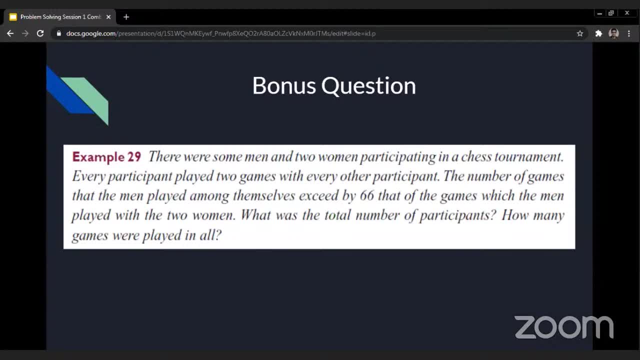 are good other questions. what I want to tell you is: just do what, like we had done in the earlier question, use some variable. okay, I'm waiting, I'm waiting, don't worry. that's absolutely right, Imran. so if I don't give out another hint, hey, do you all want me to give out another hint? if, if you? 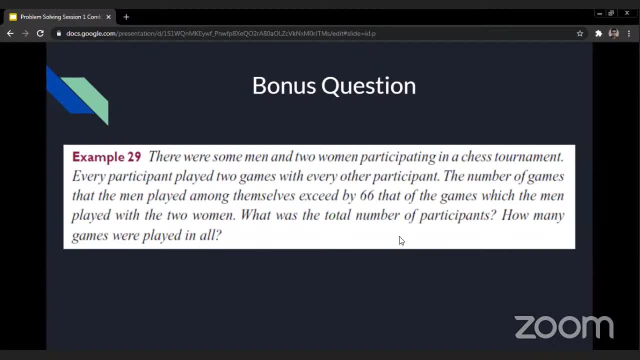 all want me to give out another hand, then you can raise your hand. let's see if more than three or four people want me to give a hint. oh, okay, okay, I won't. I won't give up the hint. let's wait for some time. after that I'll give up the hint. I want the other people to take more part as well, there. 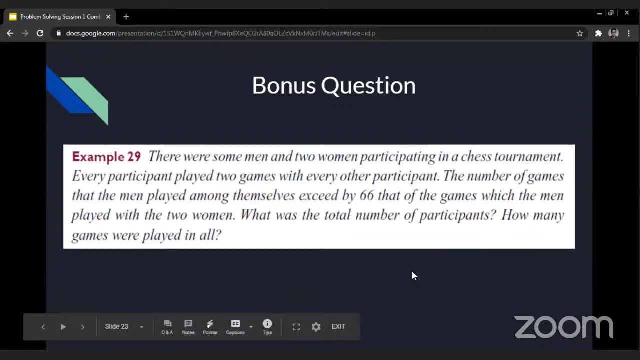 are some people who are giving non-sense continuously. but it would be great as okay, okay, okay. so I guess that would be right, Imran, but I am not really sure about the numerical value because I haven't memorized it. actually, I, it's on the next slide. 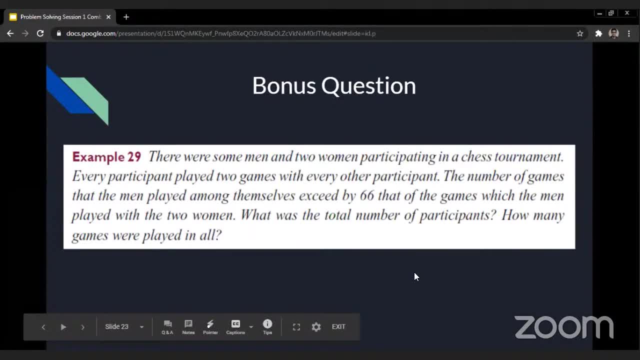 we'll see. let's see another minute or two maybe, and after that maybe I'll ask you guys if you need a hint. you can't continue like this forever, right? okay, I'm giving you guys a minute or two to solve this. take your time, because this is not such an easy question. you can use variables. the hint is to: 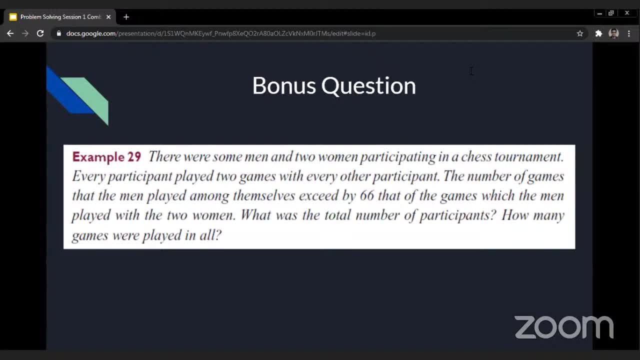 use variables like we did before, take some X or take some a or take some n or anything like that, and try to construct, try to think of how you can construct such a tournament and how, how you can find a total number, and all because one one. another small thing I want to point out would be that we 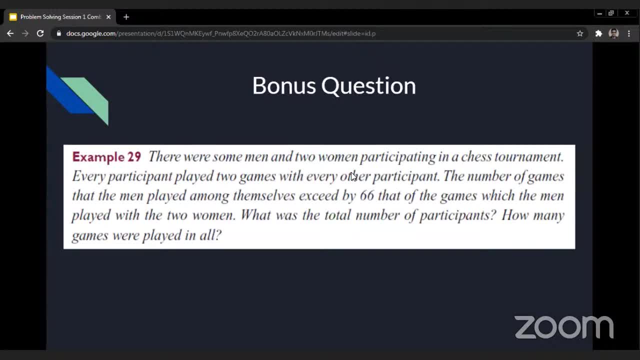 are given there were some men and we are given there were two women. so this is one thing that I just want to point out. hopefully that will help you guys. if you have any questions, or if you have any questions, please feel free to ask them in the 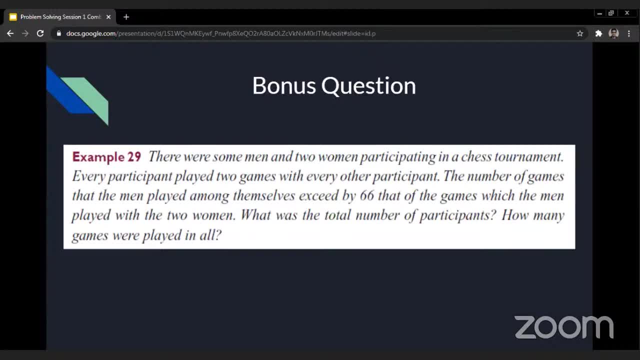 you, you, you. so i'm still waiting for answers, okay, okay, so i've got, uh, one answer, that is 11, 11. okay, write somewhere. okay, so i'll wait for some more time. uh, if any one of you have anything to tell, then you can type it out in the chat and 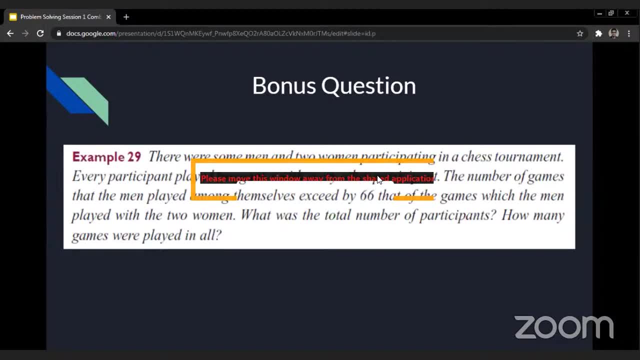 uh, after some time we'll just give out the solution to this bonus question and then we'll end the class. uh, okay, okay, okay, sure, write somewhere, right? so i think we can move on now. i haven't received any other answer. i guess only samyak and nimran have uh. 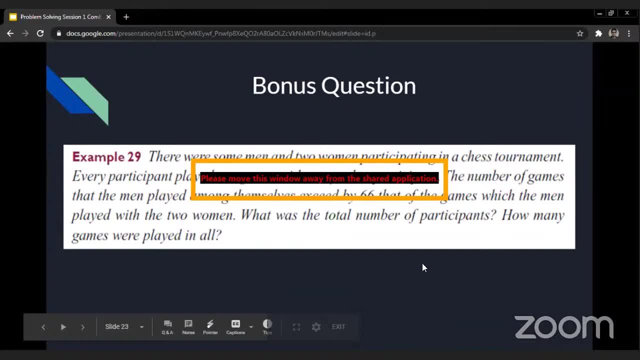 given the answer. let's see what. what happens. okay, 11, 35. let's, let's see what the answer is. okay, i i think now some of you have uh given me the answers, but uh, i'm not really sure what, if they are right or wrong. let's, let's see what the answer is. 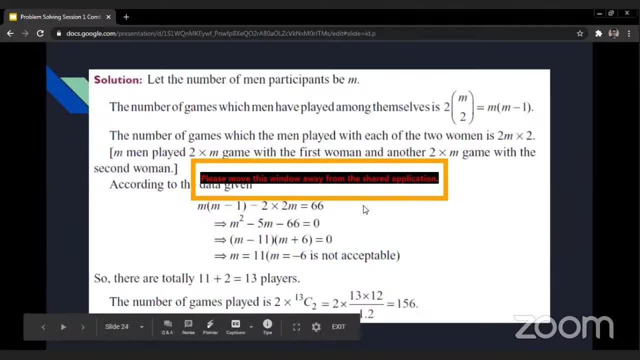 let's check it out. okay, samyak, what you had given me is exactly the same thing what is written here. okay, so what you get is a quadratic, and how you get it is due to logic, because, uh, we have m okay. okay, we have m for m. 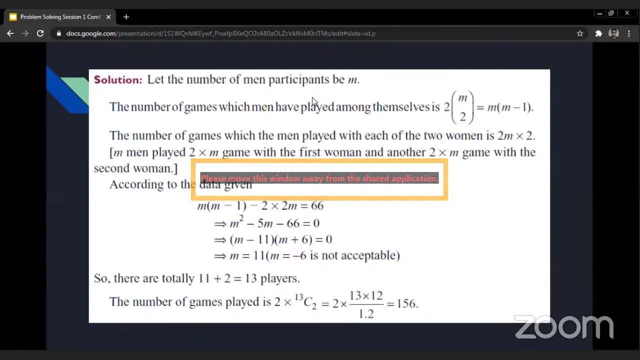 and uh. okay, i had given out this bugin because you have to take some men, so let there be x or maybe mn. the number of games which men have played among themselves is two times m. choose 2, which is m into m minus one, and the number of games which the men have played with each of the two. 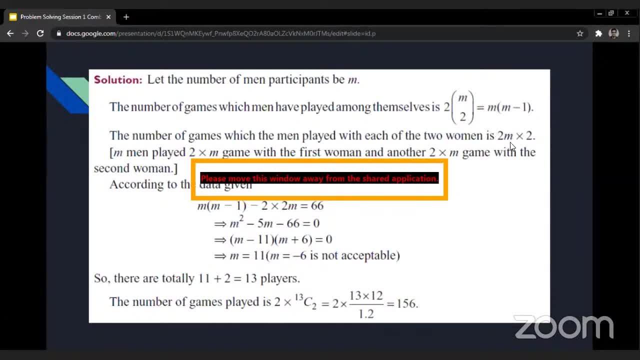 men, multiplying that by two, that is two m times two. and okay, so this is because, uh, m men have played two times m game with the first woman and another two times m games with the second one, and what we know is that m times m minus one, minus two times two, m is 66 and due to this, we get a quadratic in. 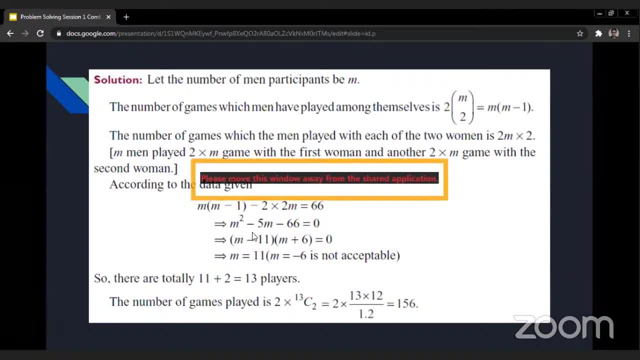 m, and this quadratic equation gives us two solutions, which are: one of them is positive, one of them is negative. as we can't have negative number, uh, we'll only take the positive number. so there are 11 men participants and a total of 13 players. how we get the name? uh. number of games. 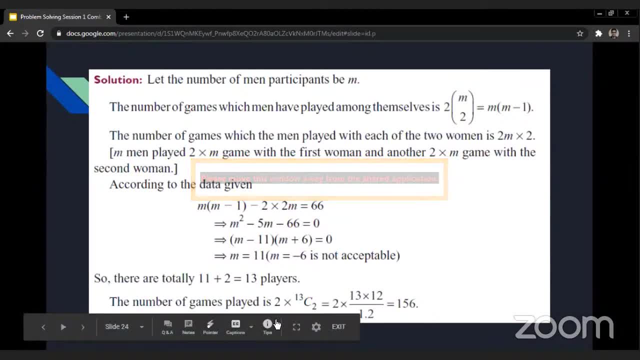 played is another interesting thing. that is just two times 13. choose two. so we choose two players and we multiply that by two, which is two times 13 times 12, by 12, which is 156. this is actually one times two you, and so the final answer is 156, and i guess many of you have sent me the answers. but 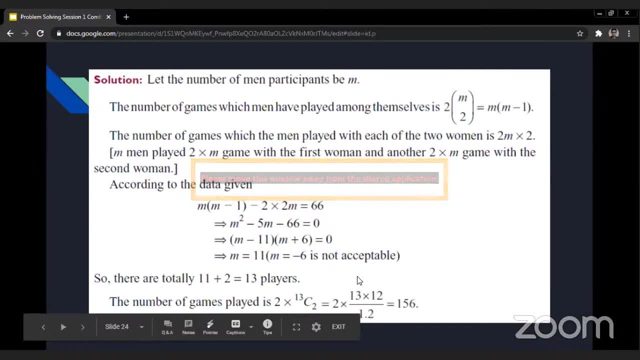 13 players and 156 games. uh, yes, this was a really nice problem and uh, thank you. uh, so such problems are quite, uh, uh, come quite handy to whenever, uh, you are attempting olympiad problems. these, these are some stereotypes which you should be knowing, samye. what do you want to tell us? 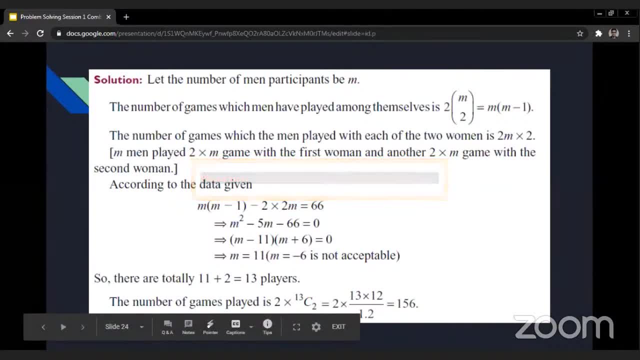 uh, yes, i would like to tell a good, great fact that on the question that find the sum of all numbers here we can use another formula. imagine we have have n digit number n is yes n digit number n is less than equal to 9. yes, n is less than.